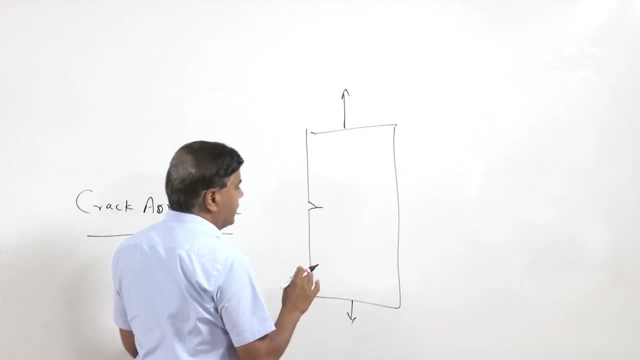 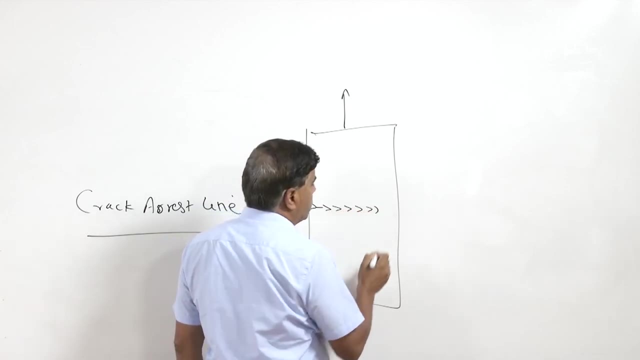 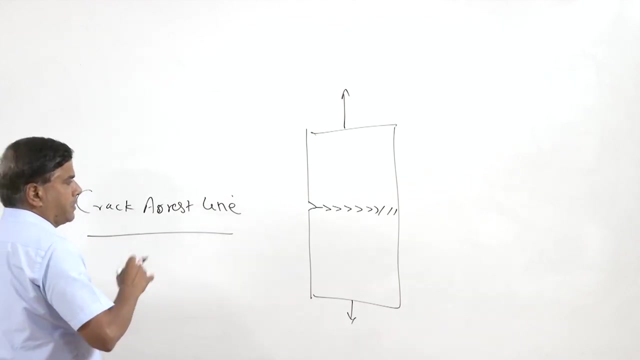 of the external loading. depending upon the type of the material and the loading conditions, the crack will be growing in different way. So when the crack grows, So when the crack grows and thereafter certain fracture takes place, what we see, the features which are obtained on the fracture surface under the static, or we can say monotonically, 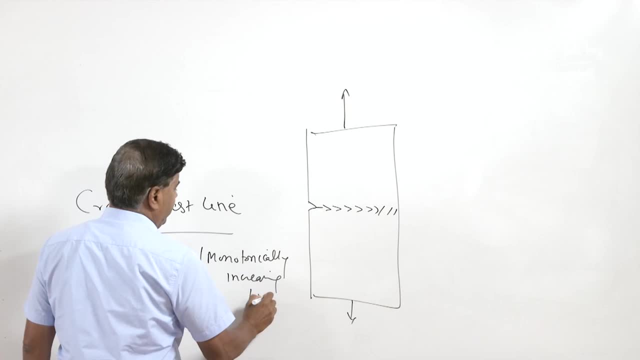 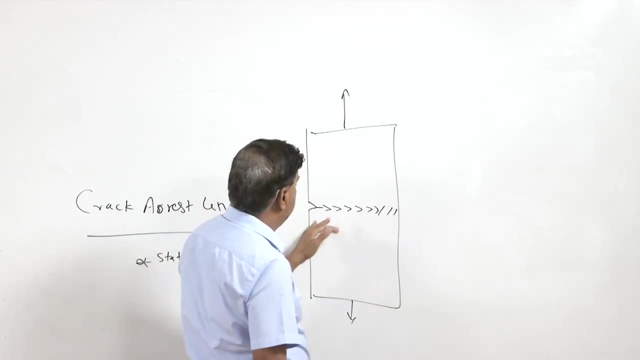 increasing load. So this is one type of the loading, like, say, in presence of the notch, when the tensile load is applied, the crack can nucleates And then it grows in particular manner. and another case is where, like, the crack grows under the cyclic load conditions. 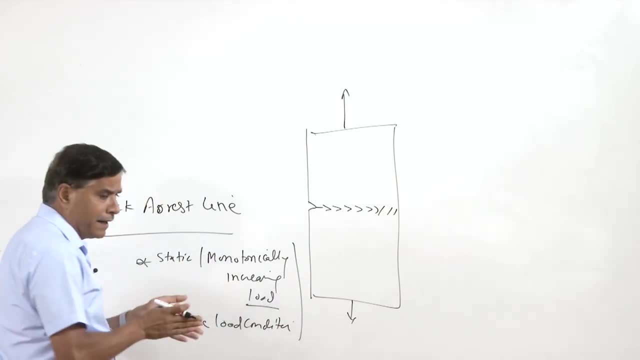 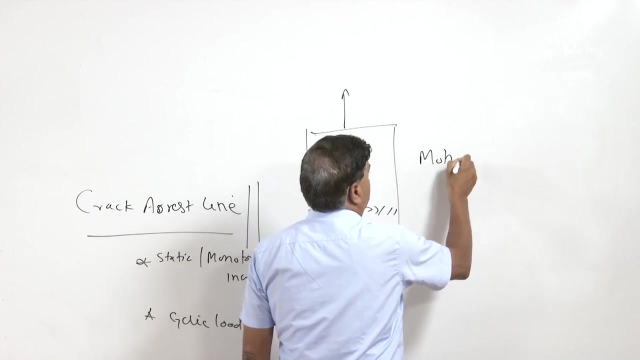 So in both the cases the growth of crack leaves some of the marks behind onto the fracture surface and those marks are termed as the crack arrest lines. So crack arrest lines in case of the monotonic loading, And monotonic loading are different than the. 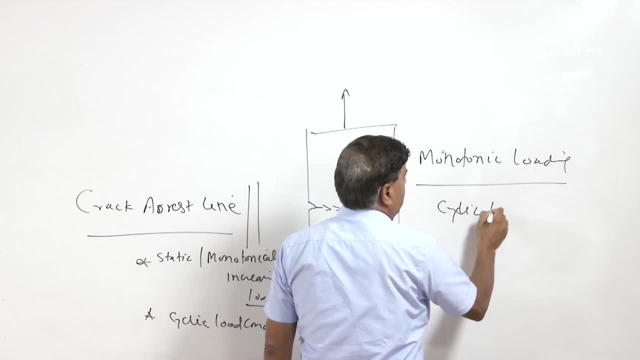 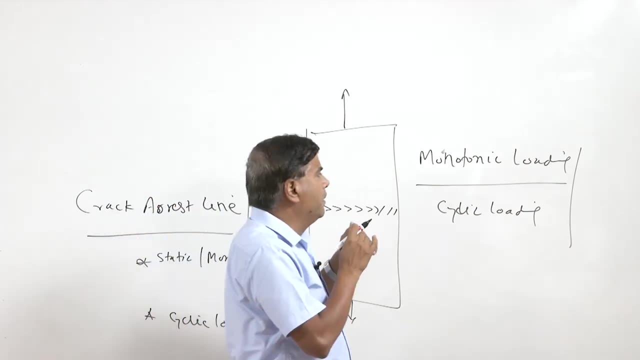 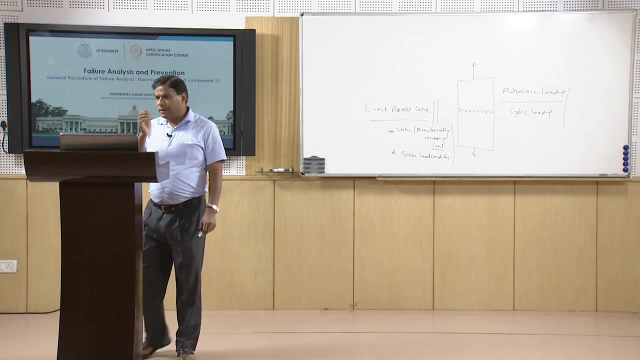 one. what is observed under the cyclic loading conditions? again, the kind of the, the stress, a state which is present. that also offers some indications through the presence of the crack arrest marks. When the crack arrest marks, under the monotonic loading conditions they are of the typical. 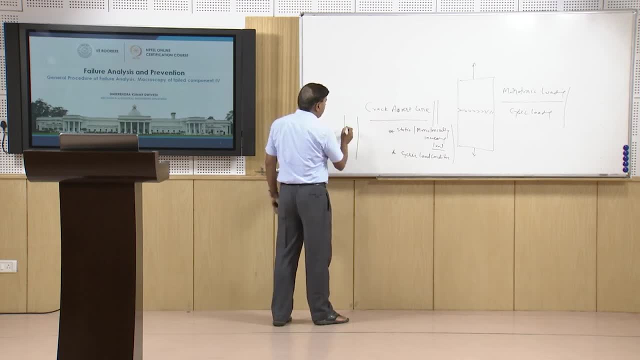 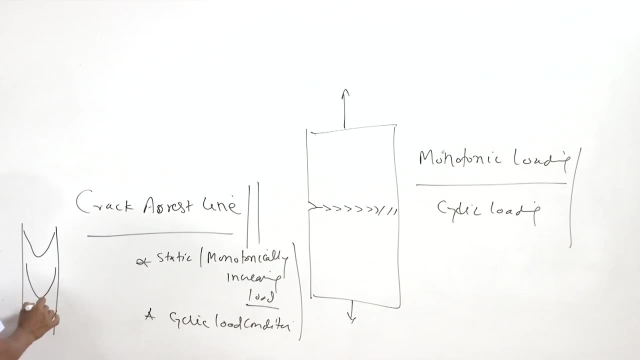 kind. This is one the thick plate. so here the crack arrest marks will be there in the U shape like this. So the tip of the U is offering the direction, in which direction of the crack growth, So obviously the direction opposite to that of the tip indicating the crack nucleation. 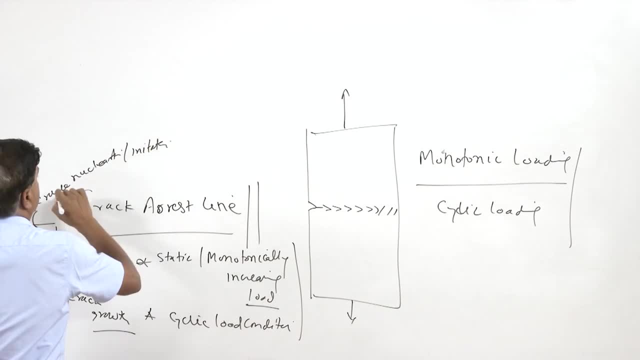 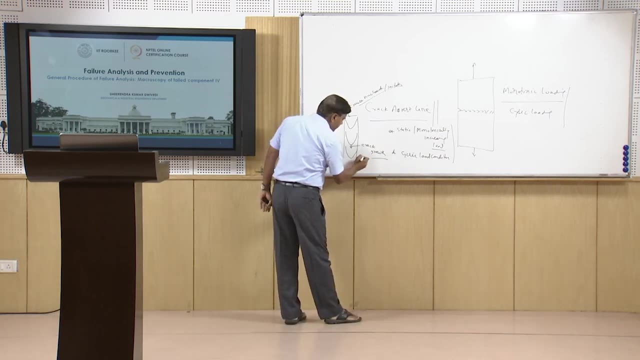 or initiation site where from it has started or triggered. So this is one case. such kind of the features are less when the plate is thick means when the plate, when the plane strain conditions are present, means it is not exactly plane strain conditions, but when the situation is approximating to the plane strain conditions. 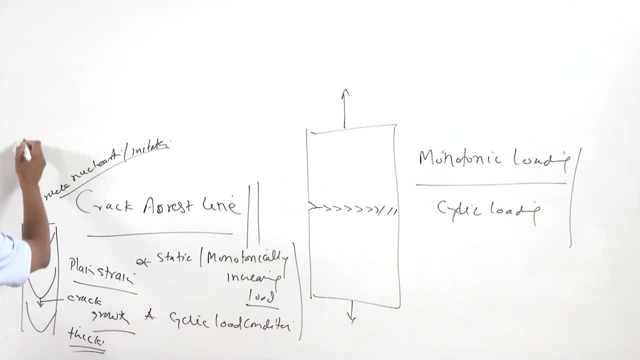 then we find a fewer such kind of marks. But when the plate is somewhat thinner we find more marks of this kind because the growth of the crack is more frequently arrested by the material and we find lot of such kind of the marks. So there are two points. as far as the crack arrest line under the monotonic loading condition, 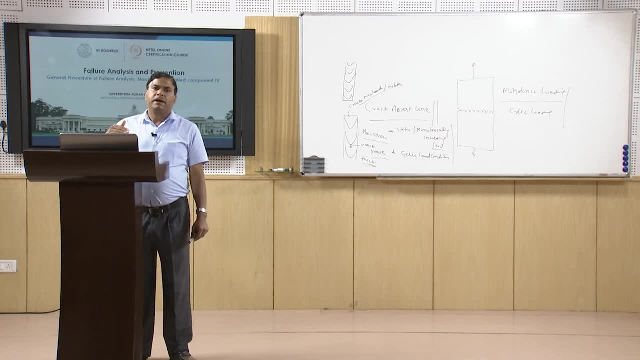 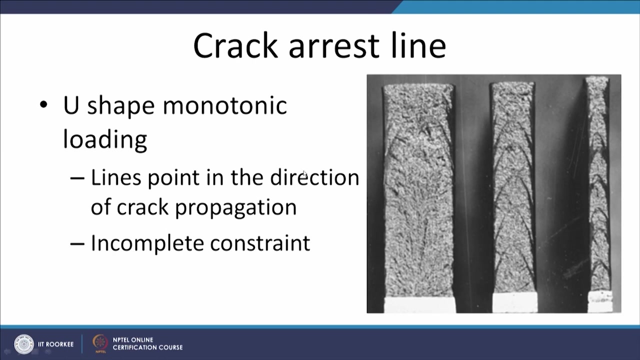 exists, that we get the U shape feature and the lines pointing in the direction of the crack propagation. So, like say, here, these U shape, inverted U shape lines are indicating the direction in which the crack has grown. and you see, So, the presence of these, indicating the presence, existence of the incomplete constraint means. 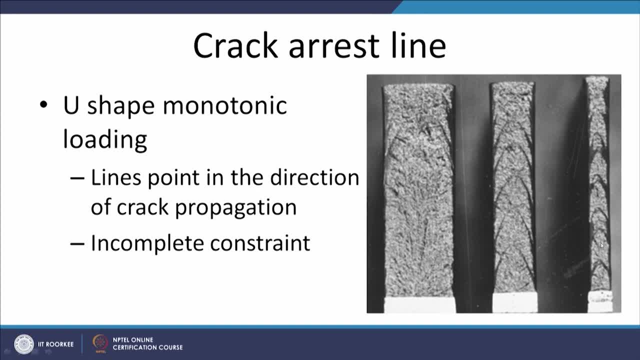 as the thickness increases. when the plate is thin, we find more such kind of the U inverted U shape marks, And when the plate is thinner, So we find more such kind of the U inverted U shape marks. plate is somewhat thicker, we get somewhat fewer marks and very few marks when the plate 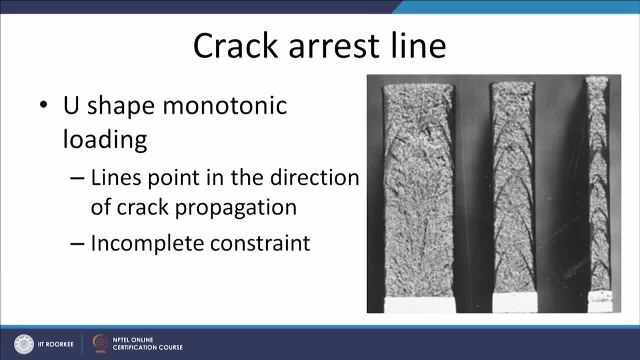 is thick, So the presence of these marks indicate that the incomplete constraint exist. and so here this is the situation: nearer to the plane stress condition, and as the thickness increases we approach towards the plane strain conditions. but still, if these marks are present, that 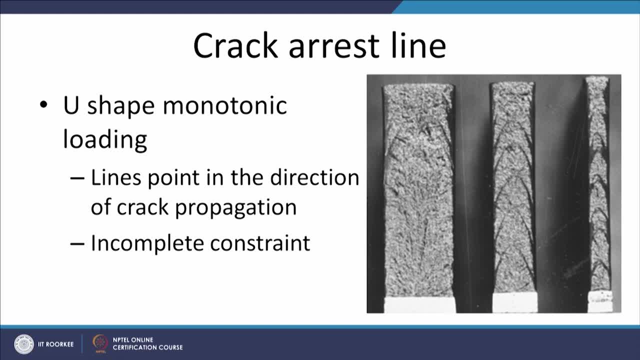 will indicate the incomplete constraint. So it is obvious that with the increase of the thickness the plane strain conditions, possibility for a plane strain condition, will be increasing and that will be increasing the constraint also. So presence of such marks indicate incomplete constraint. 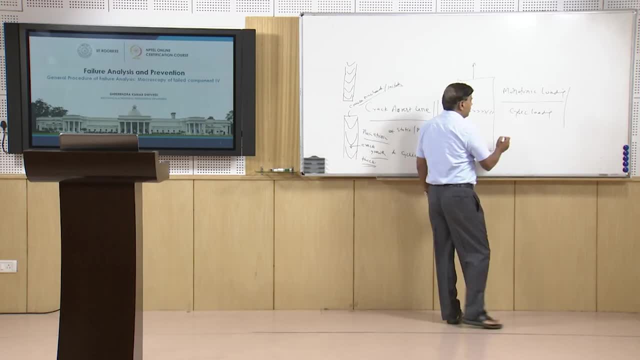 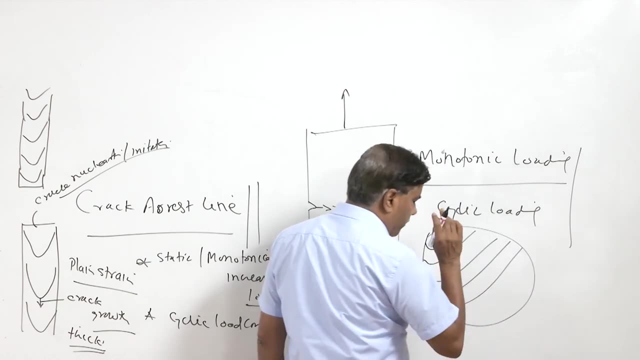 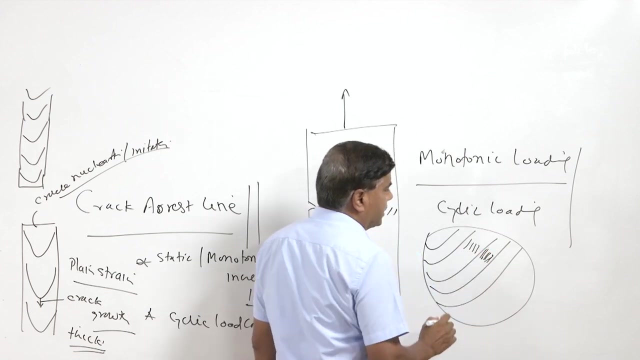 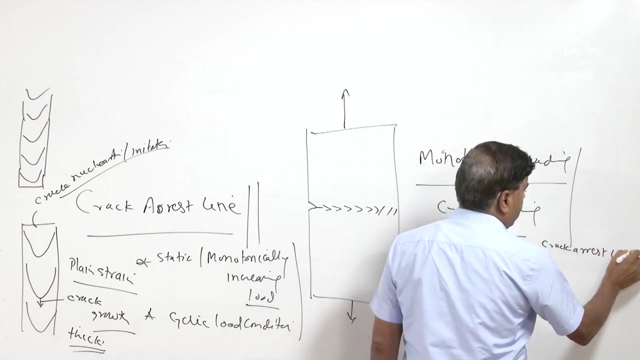 While under the cyclic load conditions, the presence of the these concentric circles in form of the beach marks or, microscopically, these are present in form of the striations at which can be seen at a high magnification. So these are also the crack arrest lines in form of the beach marks or the striations. 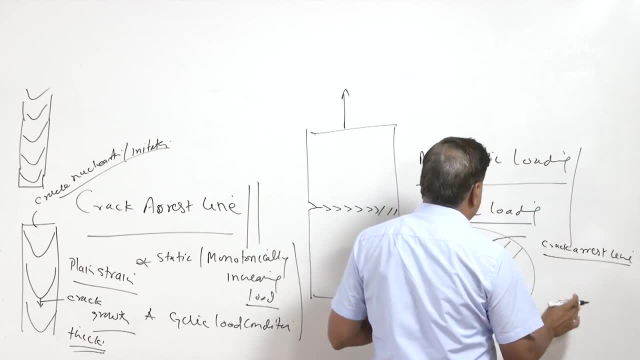 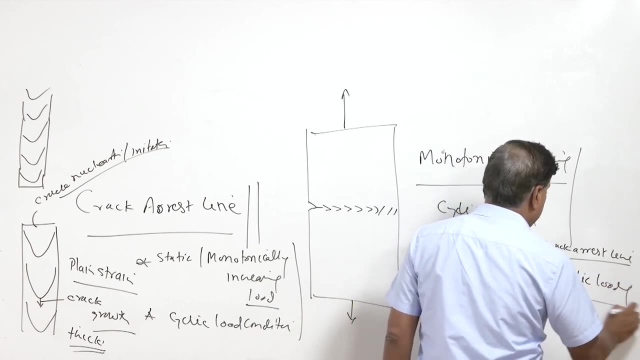 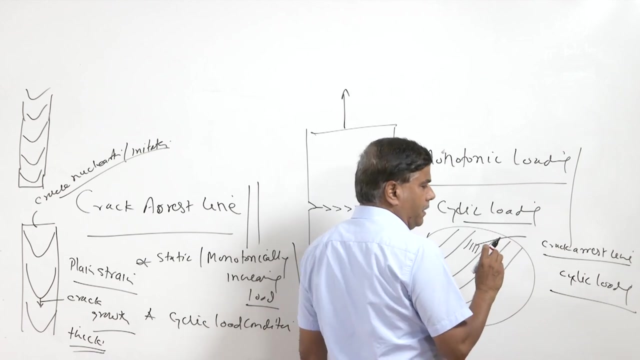 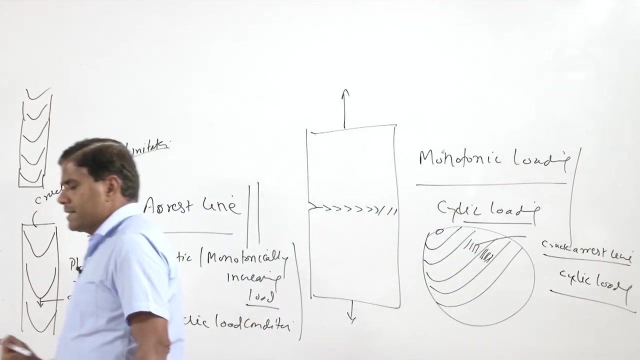 and which will be indicating the presence of the cyclic load conditions. So these are also So loading and the direction in which the crack is growing. so the circle, the centre of such concentric circles, will be the location where from the crack has initiated. 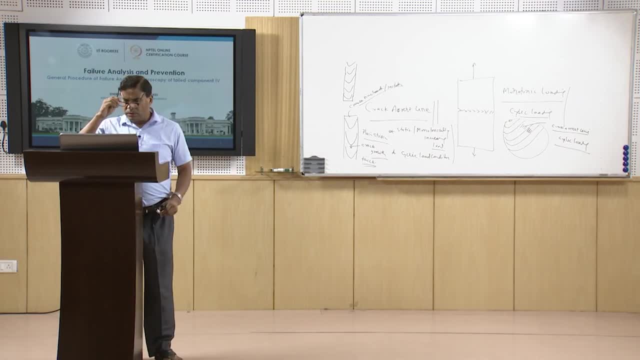 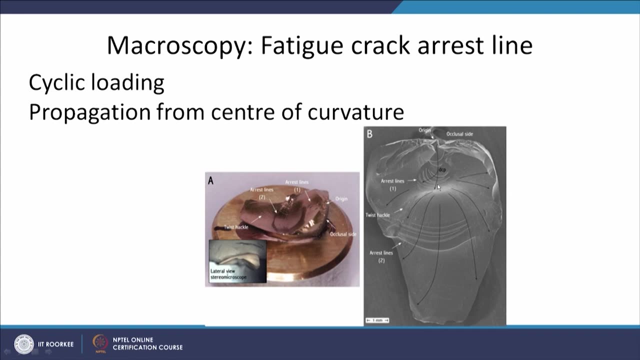 So this is what we can see in this diagram, also what it shows: that there are number of the crack arrest line in this component which has failed. similarly, there are number of crack arrest lines. So these are the lines which have failed and it is also indicating the direction in 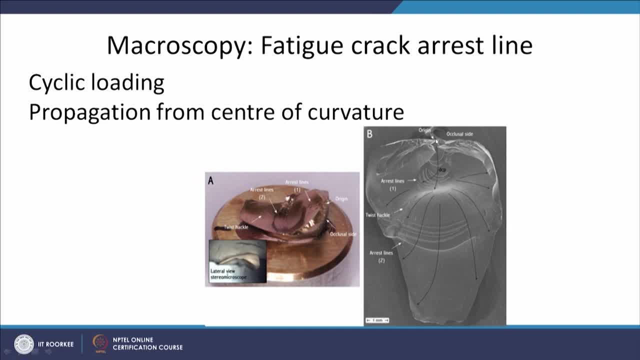 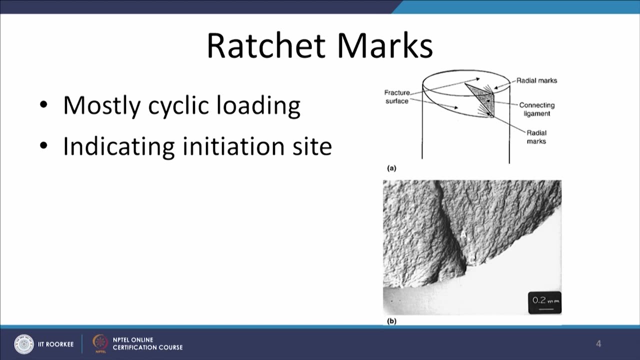 which the crack has grown and the origin is somewhere here, where from all these have initiated. So all these concentric circular lines indicating the presence of the crack, arrest marks on the fracture surface. Then another mark which indicates the fracture initiation site. So this is another mark. 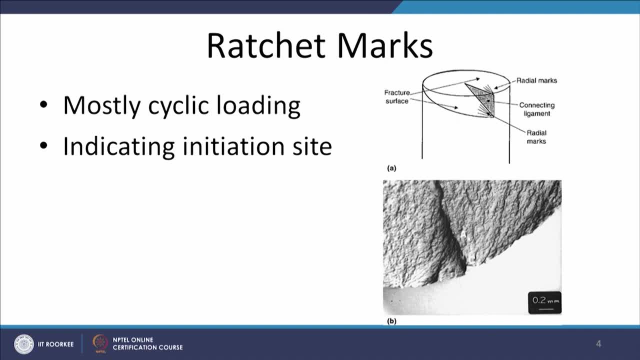 So this is another mark. So this is another mark, And this is observed mostly under the conditions of the cyclic loading, and the ratchet marks can be seen even macroscopically. this is because a very and this kind of feature can be seen. 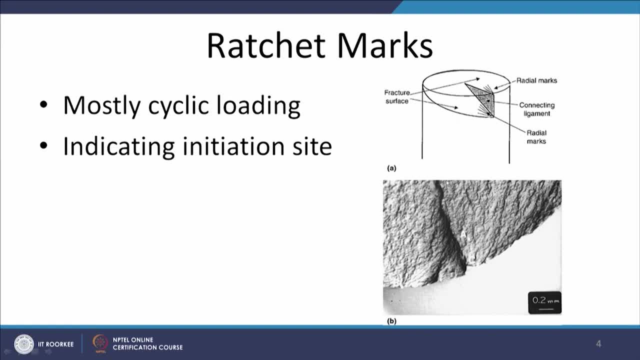 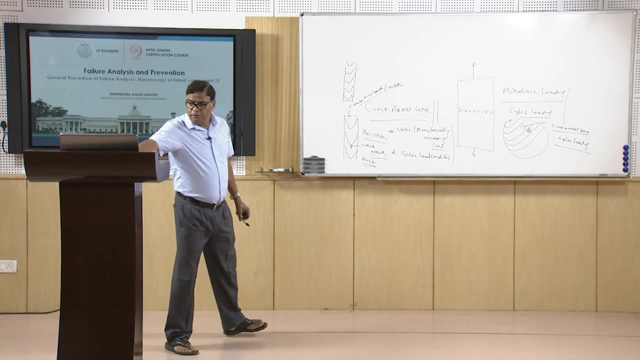 through the naked eye also, And this is indicating the presence of the ratchet marks, which suggests the site where from the fracture has been initiated And it is commonly formed under the conditions of the cyclic loading. Now we will be coming across the other aspect related with the fracture, where we have talked. 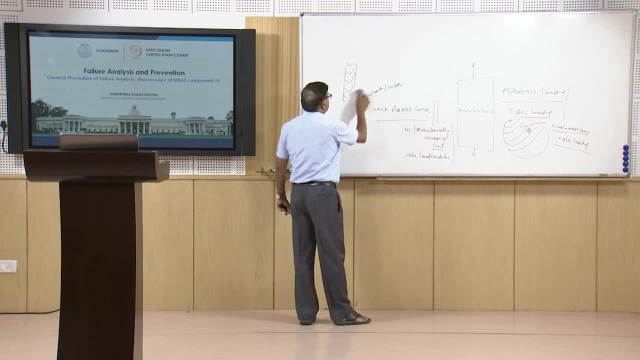 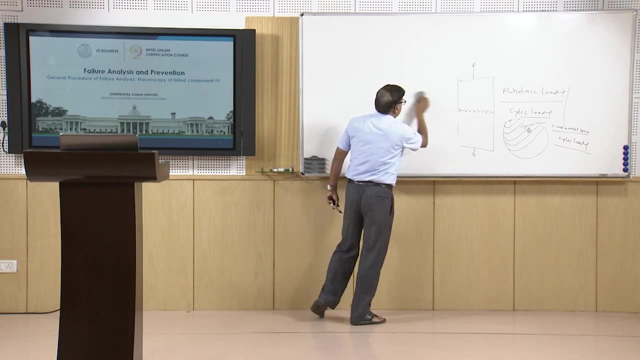 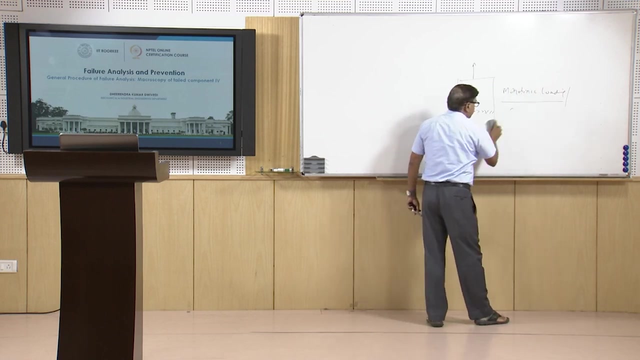 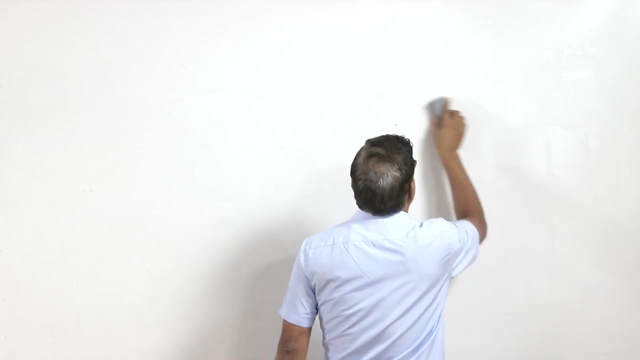 about the texture, colour and the surface roughness, and what kind of the inferences can be obtained from such kind of the surfaces? Thank you very much. So decolourisation or change in colour itself indicates either the component has been exposed to the corrosive environment or it has been exposed to the high temperatures because of 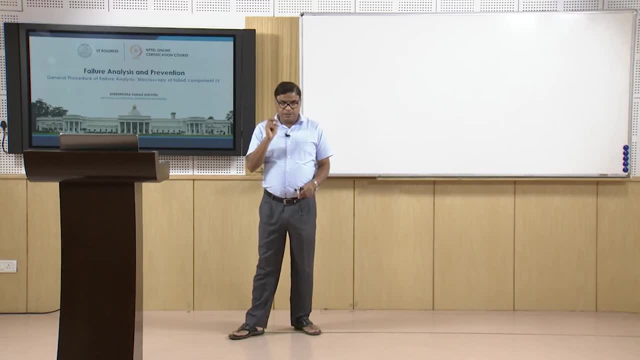 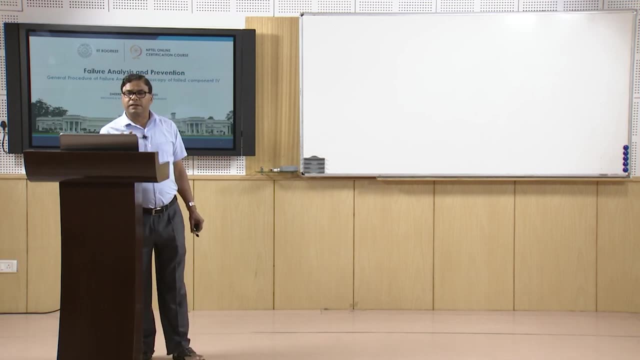 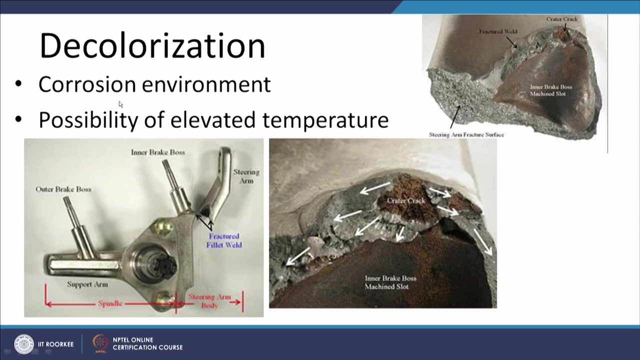 which oxidation has taken place. So these are the two possibilities. If there is any change in colour of the metal during the service, so that will suggest the possibility. these two possibilities, Let us see So like presence of the corrosive environment in which component has been exposed, or the 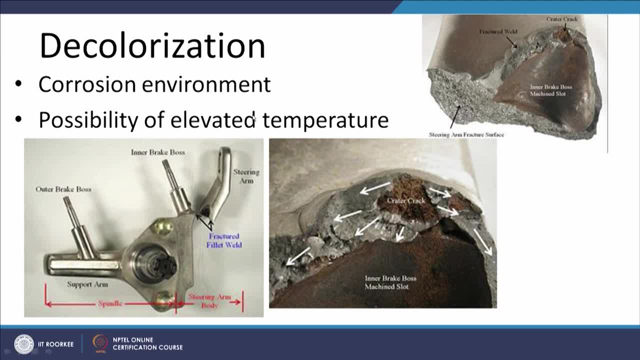 possibility of the elevated temperature, so that oxidation would have changed the colour Like say. this is one particular example where the failure had taken place of the steering arms which was welded, and what it shows: that the in the weld joint there was a crater. the crater had lot of the rust. 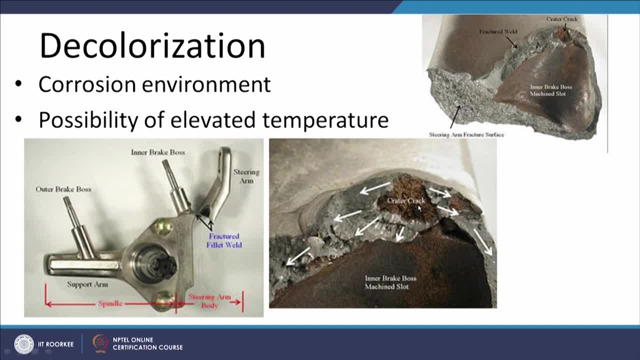 So this is the case. The corrosion features because of the different colour. this is what we can see, So the macroscopically, if we see from a distance, then what we can see. the fracture occurred from the weld zone and this is the location of the crater where we can see some corrosion. 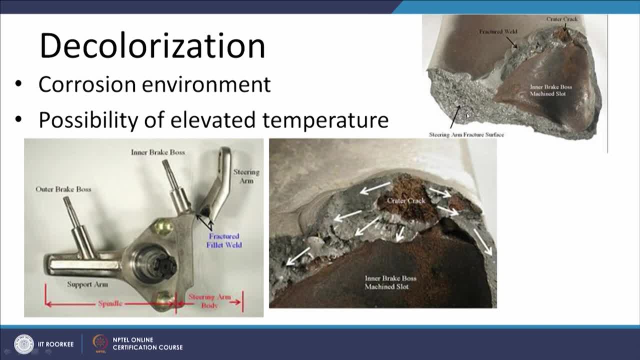 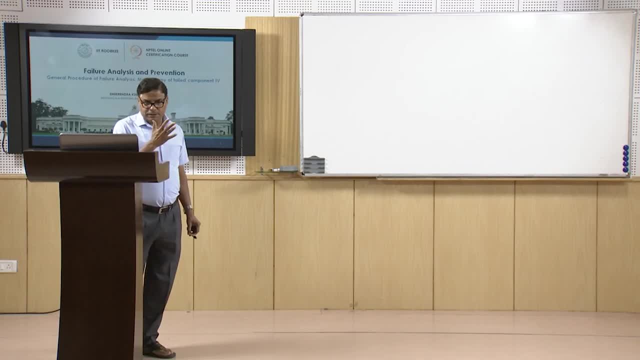 features and the bright shining surface indicates the freshly fractured surface. so it will be indicating that the surface, So the surface, was exposed to the corrosive or environmental conditions for certain period of time. with the change of colour, and if there is some freshly fractured surface, then it 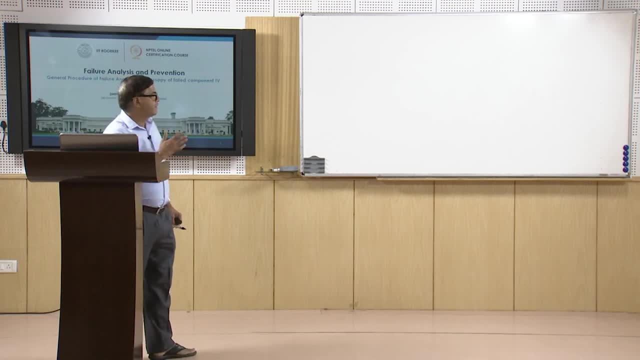 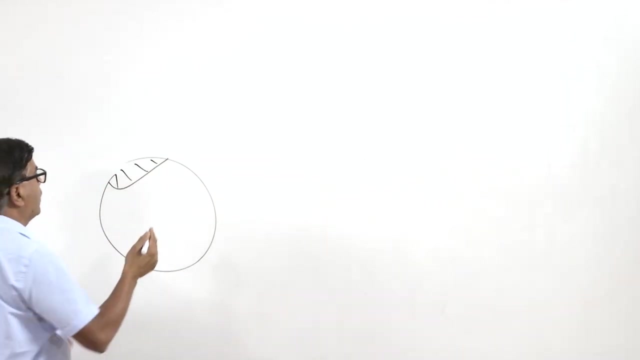 will be the bright and the shining. and the reflective means the bright in colour and it will not be dull. There is one more possibility: that if this surface was exposed in the environmental conditions for long, then it will get oxidized, and the another one which will be failing catastrophically. 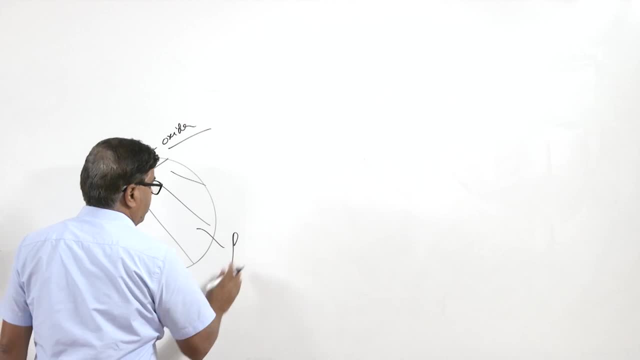 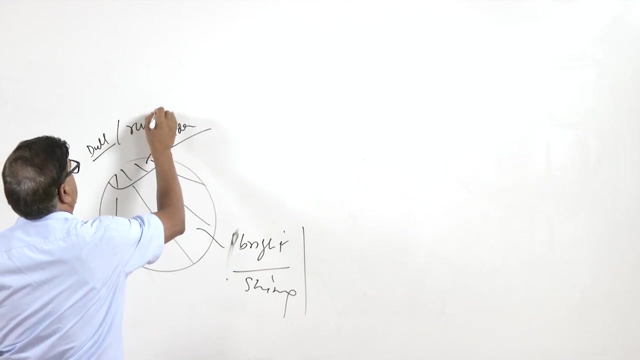 under the overload conditions, so this will be comparatively bright and shining. so this will suggest the possibility of the freshly fractured surface, while if the when a particular region where we can see that it is dull And there is a presence of oxide or rust as per the metal, it will indicate it has been 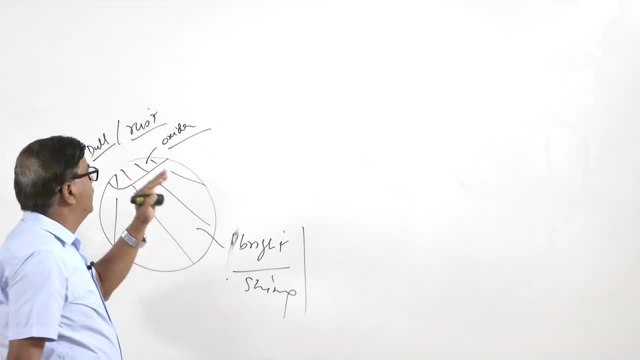 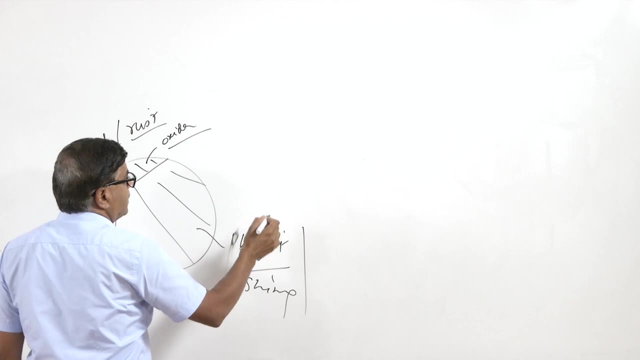 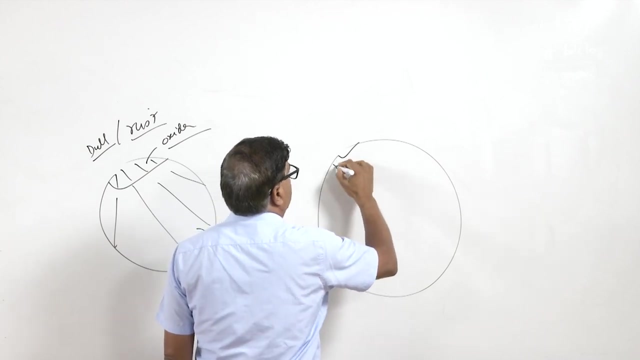 there for certain period of time, because of which rusting or oxidation has taken place. There is one more aspect, which is that by measuring the thickness of the oxide, like if this is the crack which has nucleated and then it is growing slowly, like this: 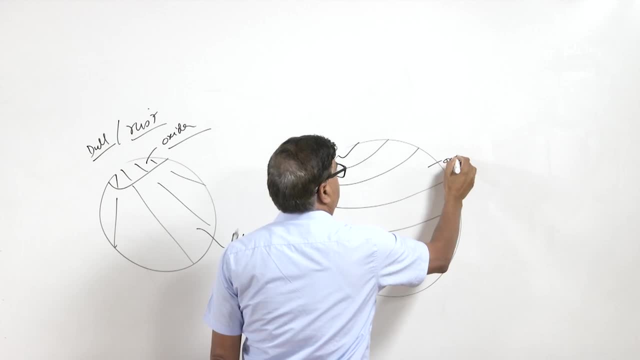 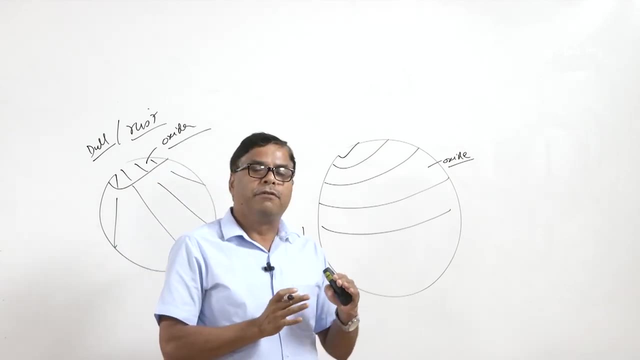 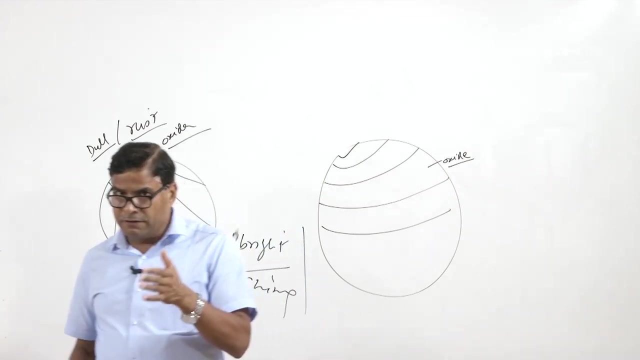 by measuring the oxide thickness layer and using the oxidation kinetics of that material, we can estimate for how long time this surface was exposed to the environmental conditions. So sometimes measurement of the oxide thickness layer helps to estimate the kind of the period for which the surface was exposed to a particular kind of condition through the measurement. 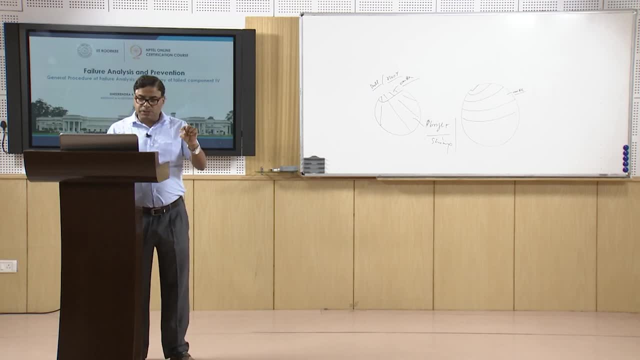 of the thickness, because once we know the thickness then using the oxidation kinetics of that metal, we can determine for how long time this surface has been exposed to the environmental conditions. So we can also see if there is a surface having the oxides, of course, in fatigue conditions. the location where crack is nucleated will be exposed for longer period as compared to the other surfaces, because the surface will be formed sequentially and the third zone will be formed suddenly in the third stage of the fracture. So the obviously the oxide thickness layer will be maximum here and then it will keep. 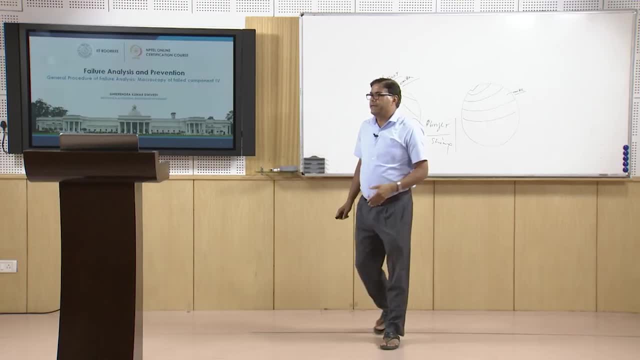 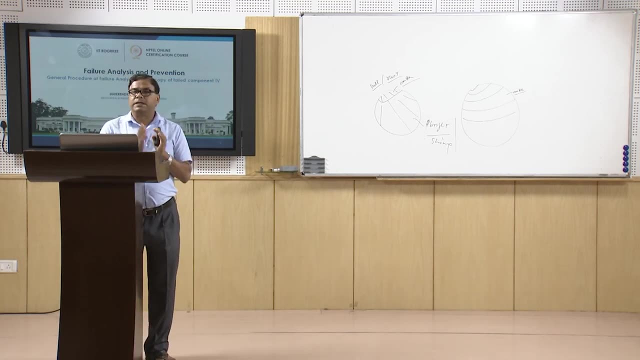 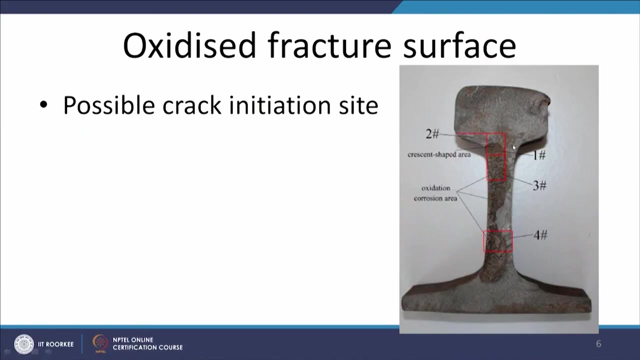 on decreasing because of completely shorter period of the exposure to the environmental conditions or the corrosive environment. So means the decolorization is there. Corrosion indicates either oxidation or the corrosion or exposure of the component to the corrosive conditions. Then oxidized fracture surface also indicates that there are two possibilities were related. 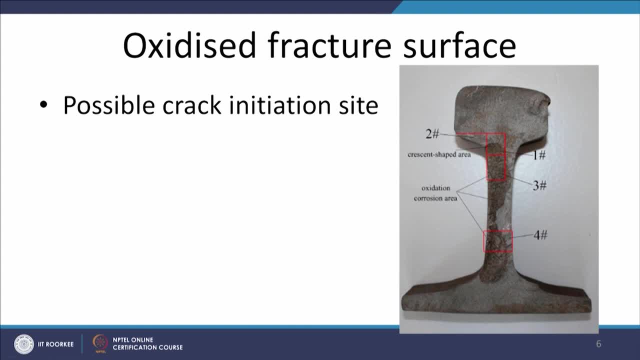 with the oxide oxidation or oxidized fracture surface. One is the location where from the crack has been initiated, because the wherever from crack initiates, that is exposed to the environment and that gets oxidized. So if there is a dull or rusted surface, that will of course indicate the location where. 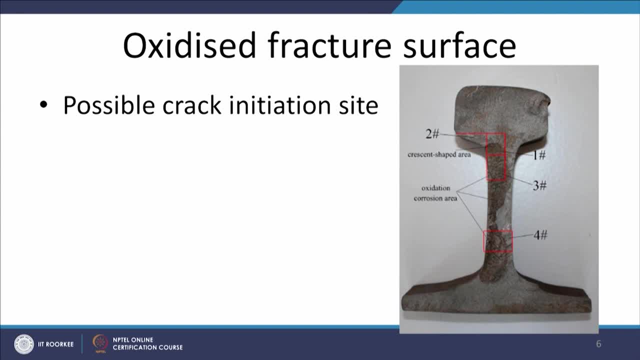 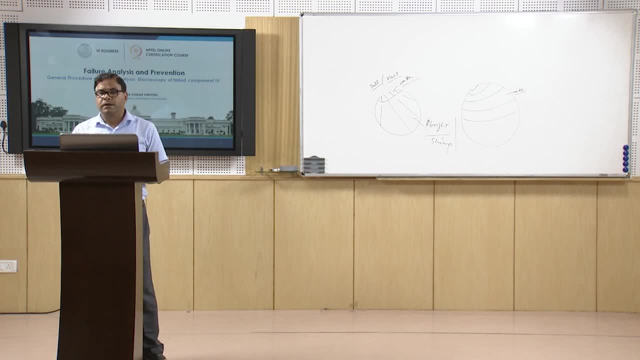 from. it has been crack has been initiated and by measuring the oxide layer thickness we can estimate when the crack was initiated and for how long time this surface was exposed to the environmental conditions Because of which oxidation has taken place. So this surface also shows. these are the freshly fractured surfaces which are the bright one. 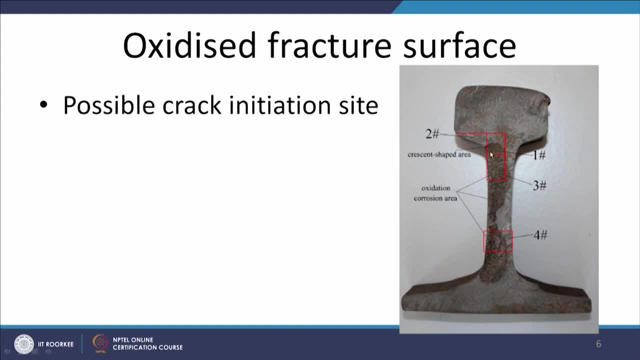 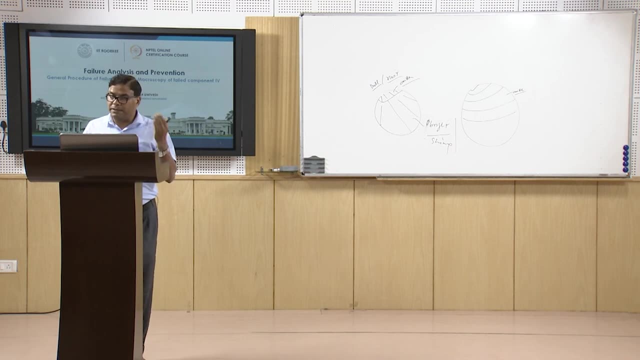 as compared to the others which are dull. So the most dull surface is this way, which is suggesting the possibility of the initiation of the crack. Other surfaces which are somewhat less dull will indicate that these surfaces have not been exposed for that long to the environment. 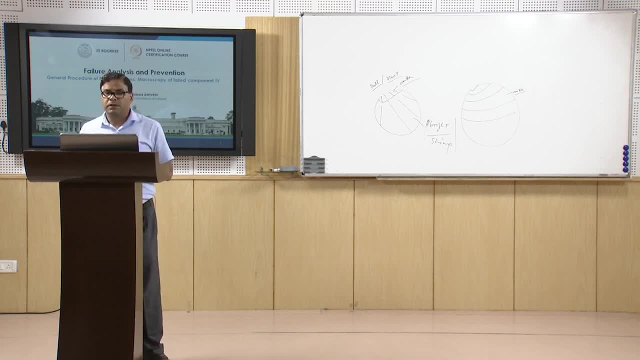 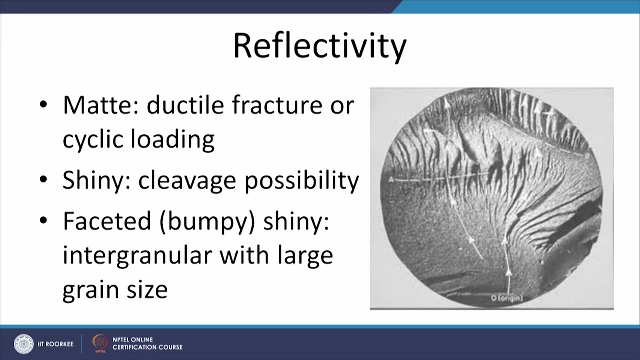 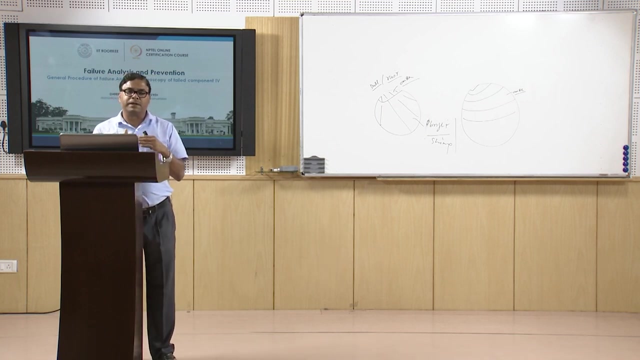 So this is the reason, So the environmental conditions are for corrosive conditions. Then another one is the reflectivity of the fracture surface. So there are few surface features like the matte fracture surface, which is which we can observe under the two conditions, when either the material is ductile, 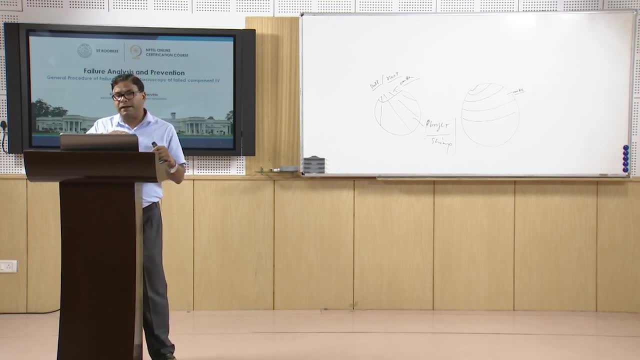 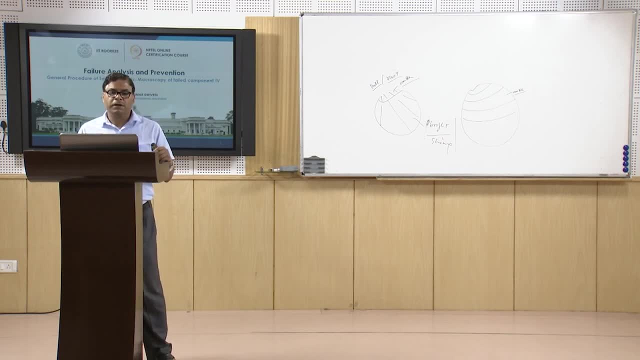 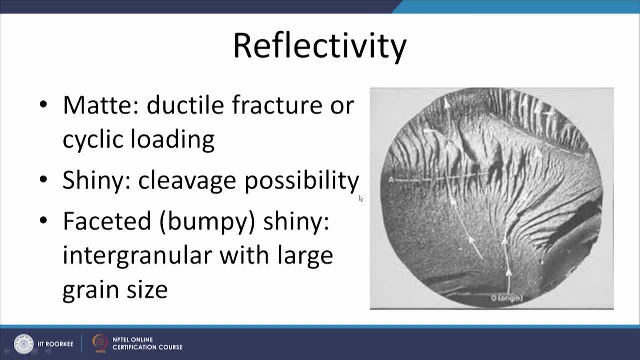 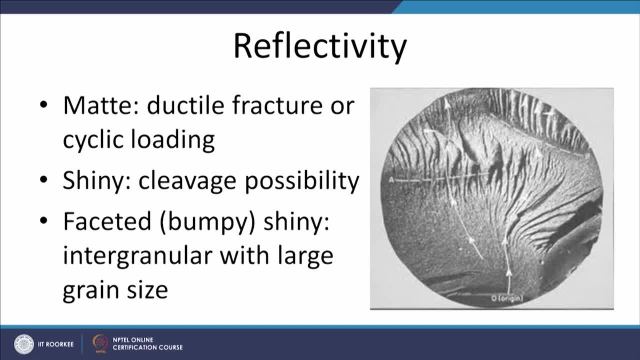 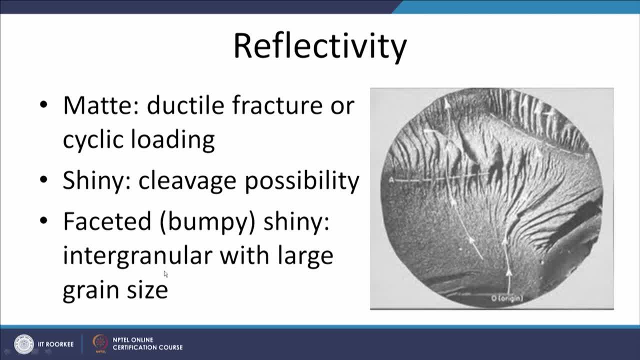 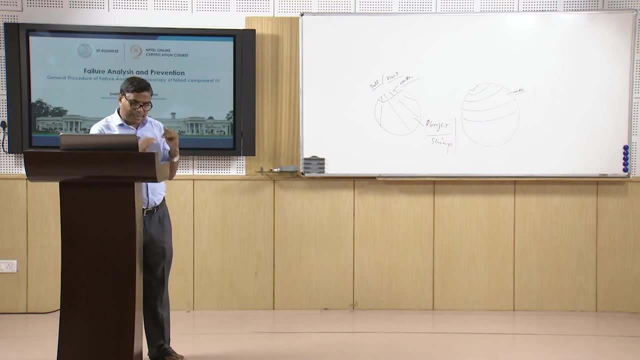 bumpy shining surface indicates that the fracture surface has been intergranular and with the large grain size. So basically these two are the common features. the matte surface indicates the ductile fracture and the shining surface indicates the brittle fracture which occurs to the cleavage micro. 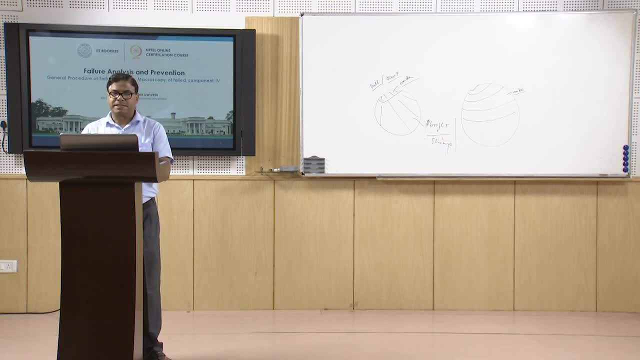 fracture mechanism and faceted shiny surface indicates the intergranular fracture with the large grain size, And a lot of information can be obtained from the surface roughness of the fracture surface. So for that what we need to see, We need to see just this diagram. 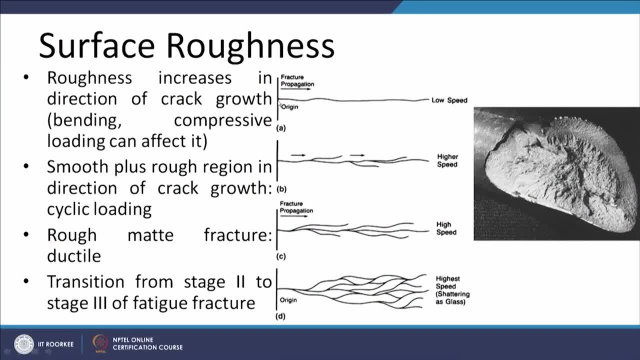 And like say, this is the origin for the crack, origin of the crack nucleation, and it grows gradually with the time at low speed. then the surface is very smooth and ups and downs are less So in the direction of the crack propagation from the origin to the end of the end, where 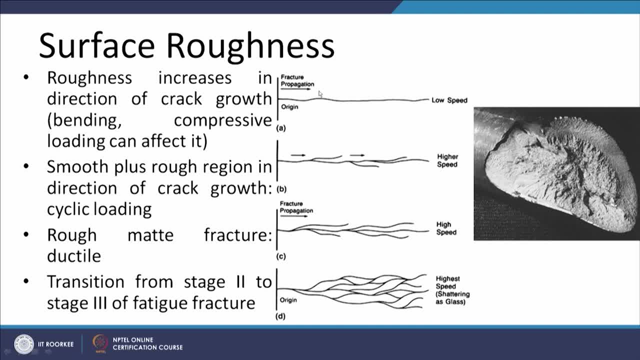 the complete fracture is facilitated. The low speed fractures indicate the smoother fracture surface. when the fracture propagates at a higher speed, then we will see somewhat a rougher surface. and when the fracture propagation from the crack initiation or the fracture initiation side at a higher speed, then we 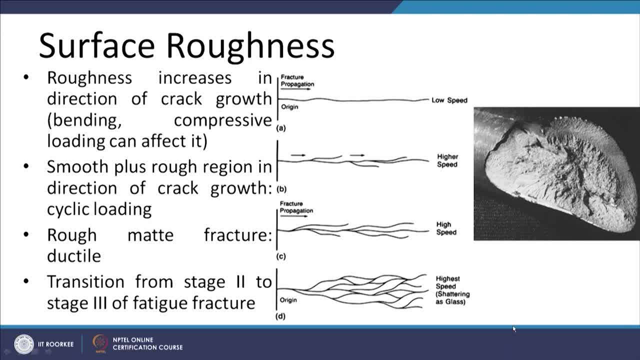 see the fracture is further Rougher and when the fracture occurs at very high speed, like the shattering of the glass, then we will see the. with the growth of the fracture, the roughness will keep on increasing. is growth of crack. roughness on the fracture surface will keep on increasing. 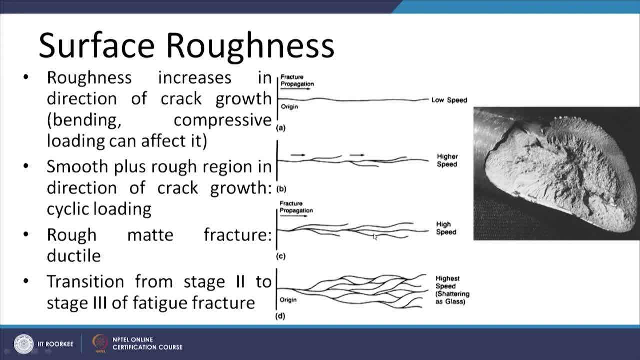 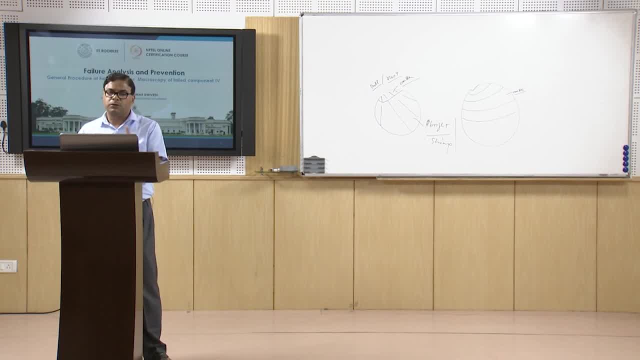 So these are some of the schematics showing the way by which surface roughness is affected. 146.. roughness is affected when the crack grows at a different speed on the fracture surface. So what we can see here: roughness increases in the direction of the crack growth. that. 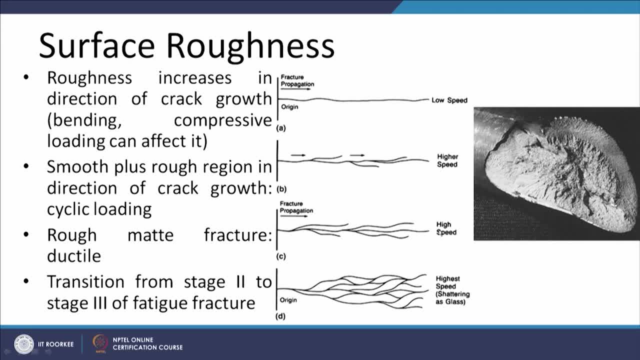 is what, except in one case, in all the cases we can see the roughness grows in the direction of the crack growth. However, the bending and the compressive load conditions can affect, because in both the cases there is a possibility for the compressive loading, so the fracture surface can get closed. 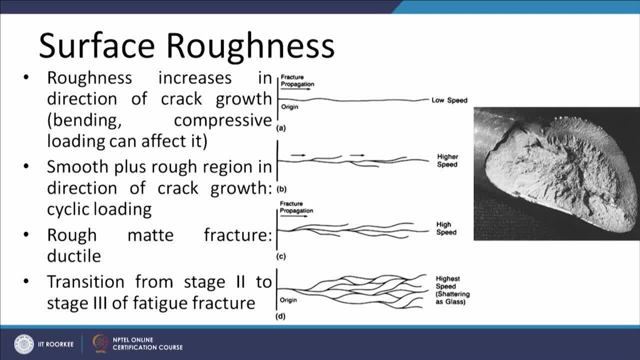 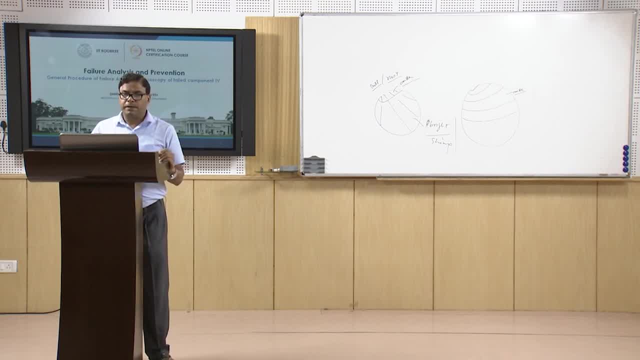 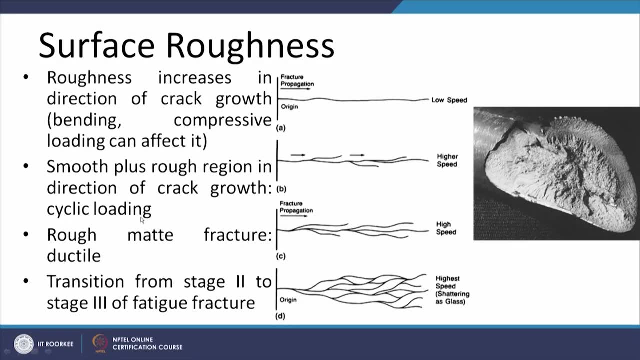 So the closure of the fracture surface under the compressive loading will smoothen the fracture surface. Smooth plus rough region in the direction of the crack growth is observed in case of the crack. So this is the cyclic loading like, say, this is what we have seen when the crack grows. 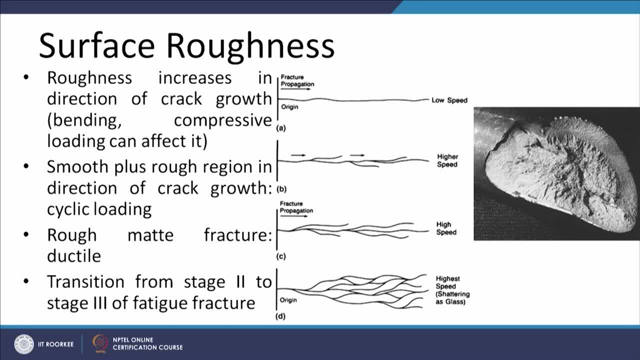 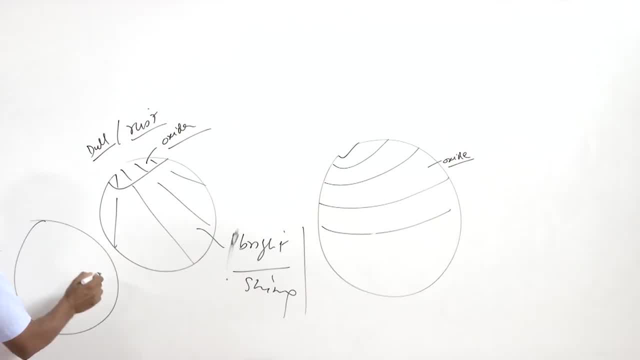 from all the direction, from the two directions, under the fatigue conditions. then we will be seeing the rougher surface will be present at the like in this case, the crack is growing from the two directions, So the rough surface corresponding to the third stage of the fracture will be at the 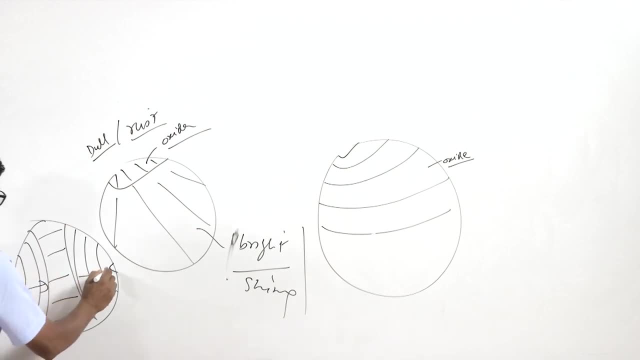 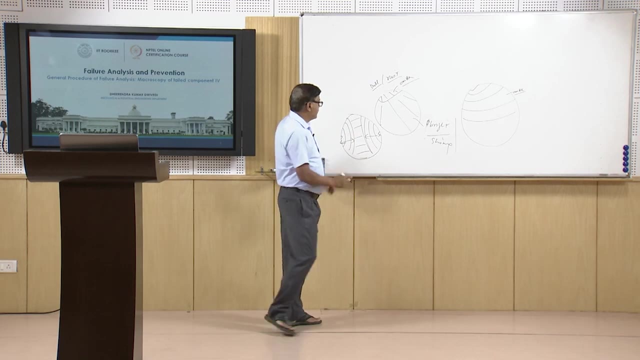 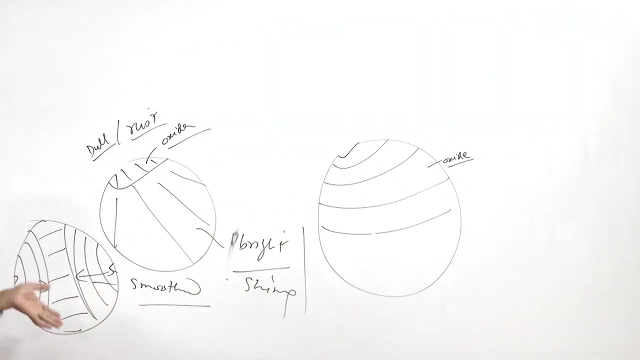 middle, while these two surfaces will be. So these surfaces will be somewhat smoother because, due to the continuous opening and closing of the crack, these surfaces will be smoothened. So smoother surfaces at the side and at the center region we may get the rougher surface. 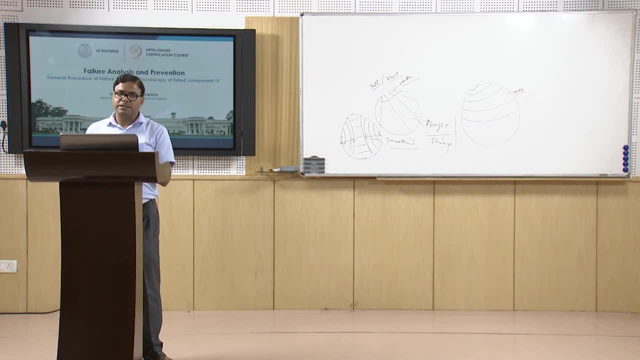 So a combination of both smooth plus rough region in the direction of the crack. growth can be observed under the fatigue load or cyclic load conditions. So this is what we have seen in case of the crack. So this is what we have seen in case of the crack. 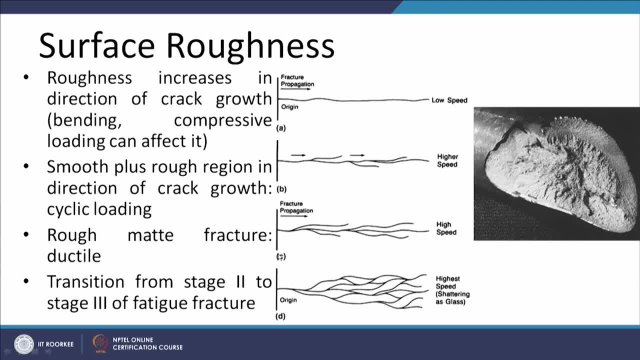 So this is what we have seen in case of the crack: Rough matte fracture surface is observed in case of the ductile fracture, while the transition from the second stage to third stage is accompanied, in case of the fatigue fracture, with lot of change in the roughness. 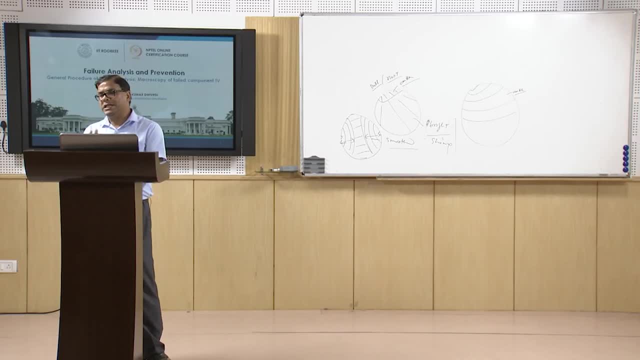 So in the second stage, surface is smooth. in third stage, surface is rough according to the mode of fracture, which may be dimple fracture or ductile fracture in case of the ductile material. So ductile material due to the overloading, or it may be brittle fracture by the cleavage. 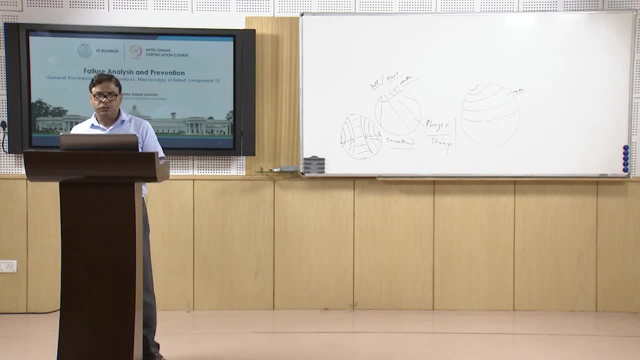 facets in case of the brittle material. So there can be lot of transitions or variation in the surface roughness, but in general increase in roughness increases in the direction of the crack growth. Now we will see the ductile to brittle transition temperature. 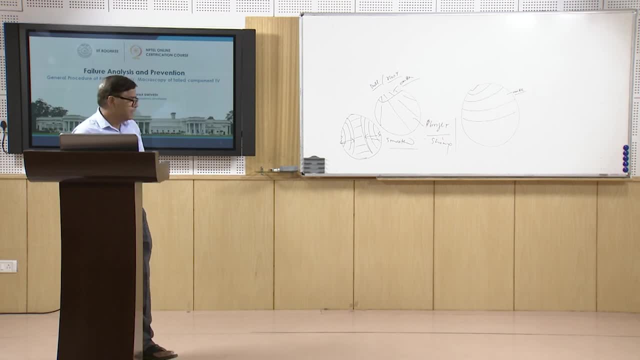 And how does it affect The fracture surfaces? So for that what we need to see. we know that with the change of the temperature of low carbon steel, there is lot of change in the impact resistance which is indicated through the Charpy or Izo test in terms of the energy absorbed. 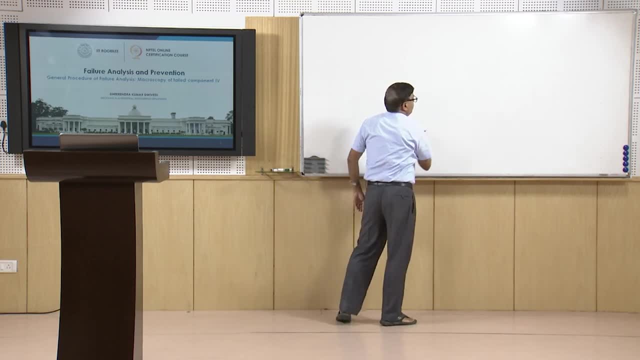 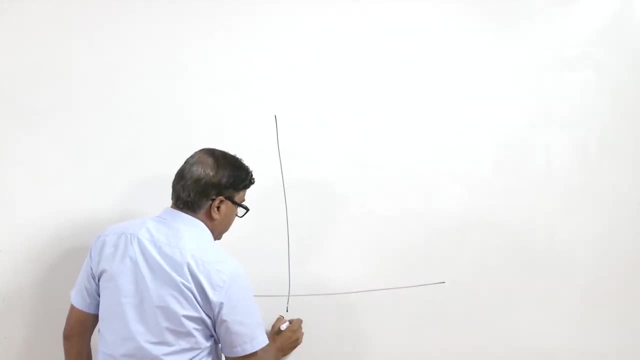 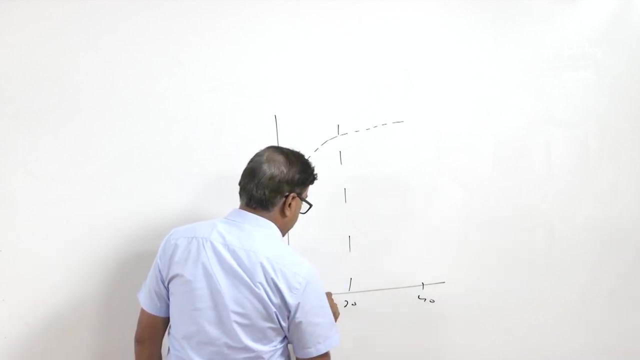 The energy absorbed may vary significantly from, say, 140.. Joules at 20 degree centigrade at room temperature, like this. so at room temperature say it is 20, then 40 and here somewhere 0, then minus 20,, minus 40,, minus 60. 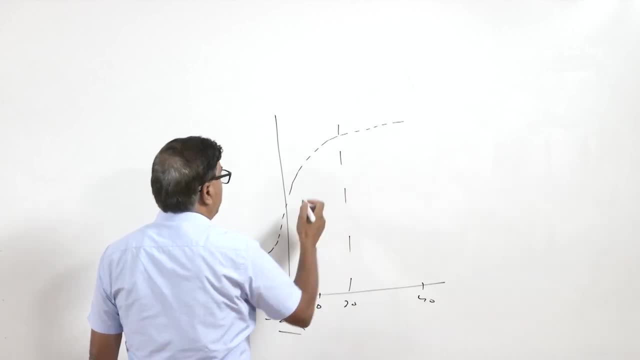 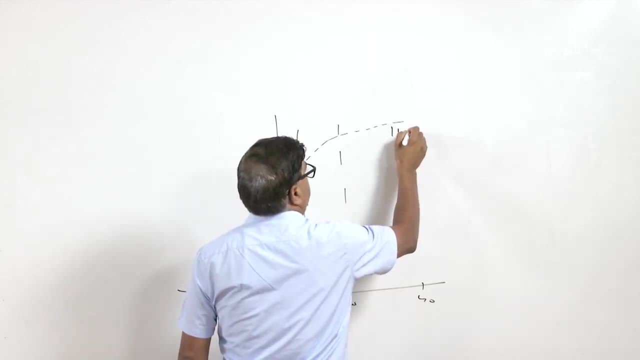 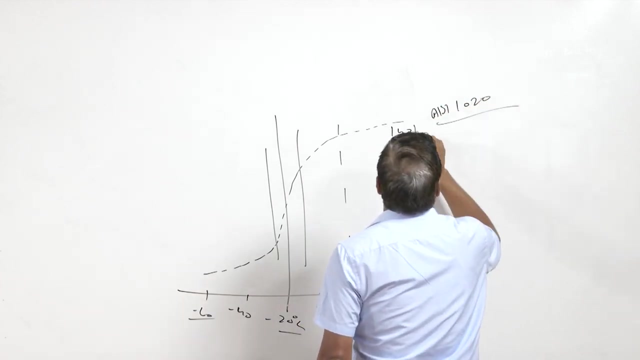 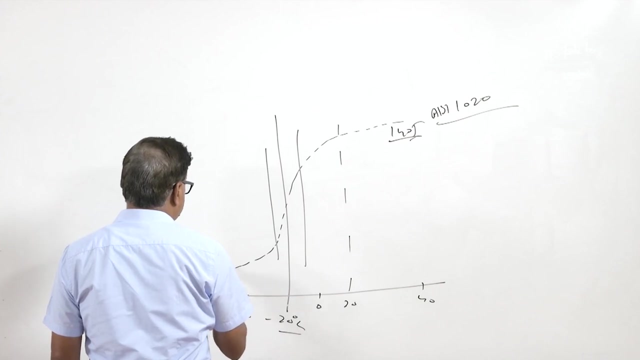 So what? it suggests? that as soon as we come down below the minus 20, there is a change in the temperature. So there is very sharp drop in the toughness value which say has been for simple carbon steel, AISI1020 of 140 joule, which may get reduced to almost like, say, the 10 to 15 joule. 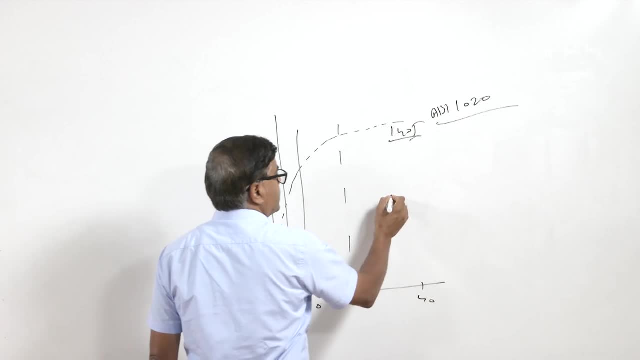 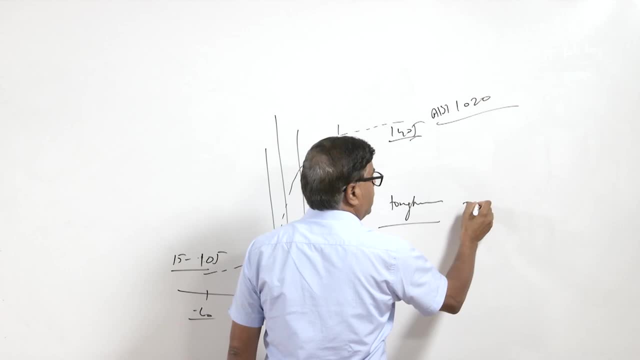 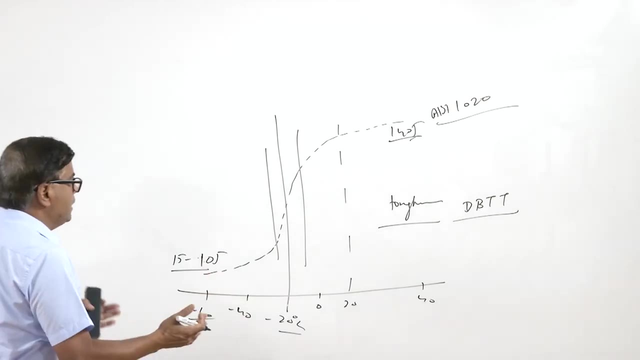 So such a large drop in the impact resistance or the toughness of the material. So such a large drop in the impact resistance or the toughness of the material. The material is termed as ductile to brittle transition temperature and when it happens, we will see lot of variation in terms of the fracture surface morphology. 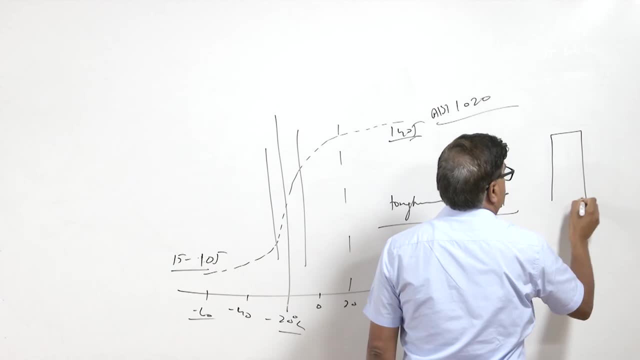 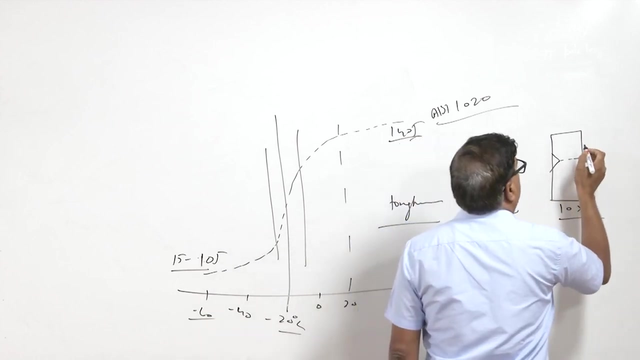 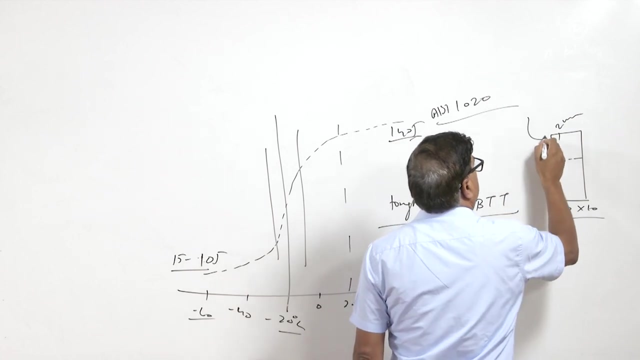 Normally our the toughness sample is of the square shape. where we make square cross section, we make a notch- 6게요 7 is normally used- and here then this is the 2 mm notch which is normally made, and then we check the impact resistance using the Charpy or Izod test. 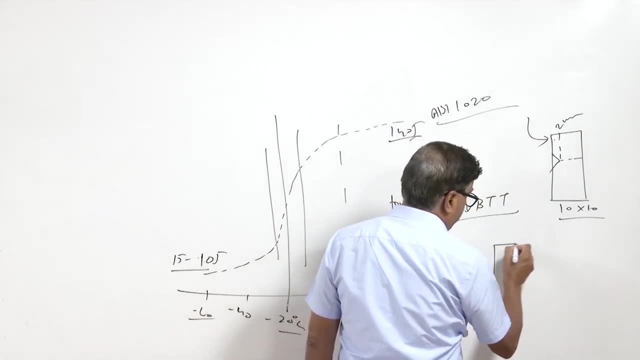 So what we normally get, like this, is the sample of the 10 by 10, so in case of the ductile materials, in case of the ductile materials, what we see? that there is a significant change in the dimension of the component, like this: 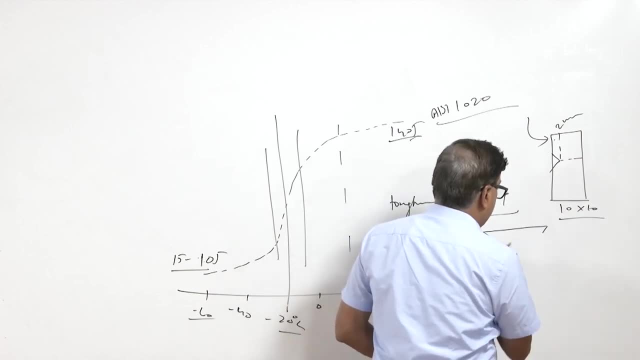 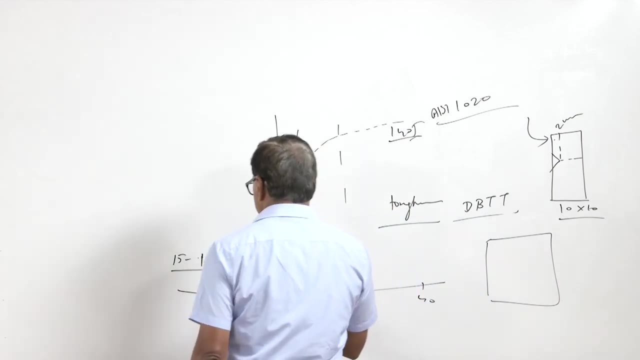 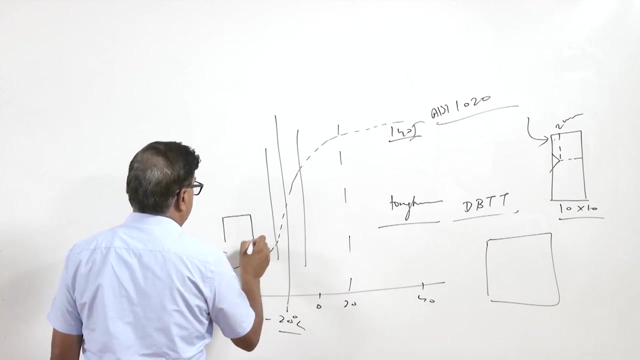 So like say, this is the fracture surface. so what we will see when the fracture is corresponding to the minus surface. So this is a 40 degree centigrade for this one. the cross section remains by and large unchanged and entire fracture surface is flat and shiny. so corresponds to the brittle fracture. 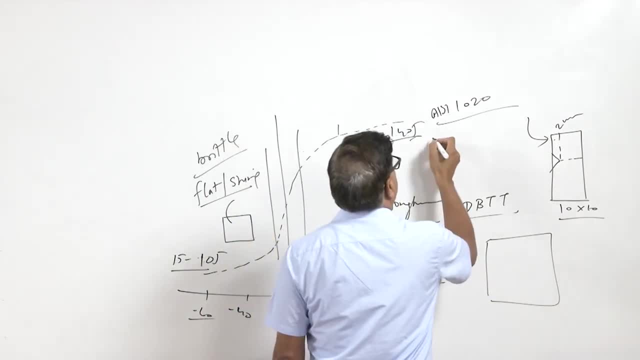 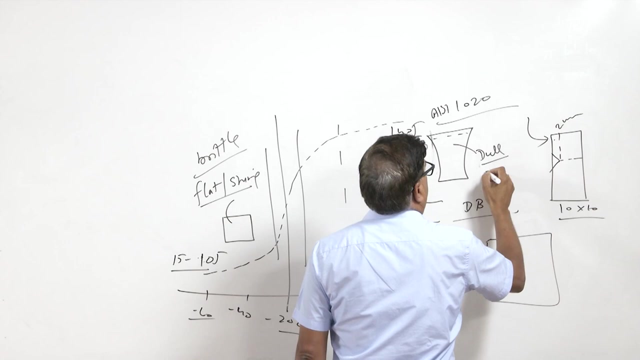 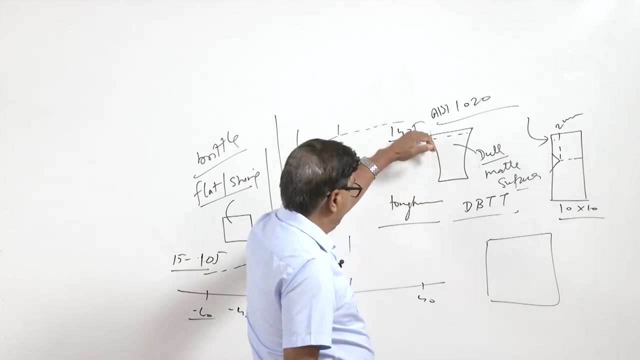 while in other case, when at a high temperature, what we see, that the fracture surface is by and large, is distorted. It is not anymore the square and it shows that lot of dull and matte surface is present. So, on moving from the high temperature to the low temperature, there is a continuous 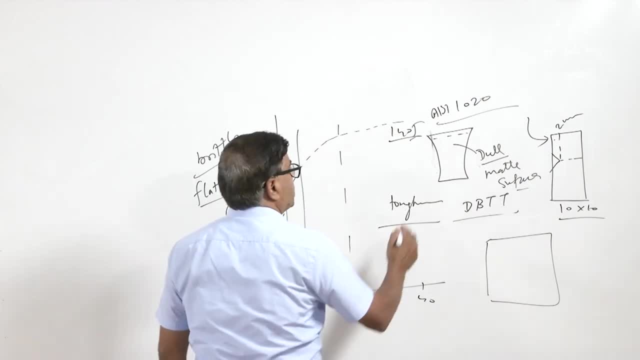 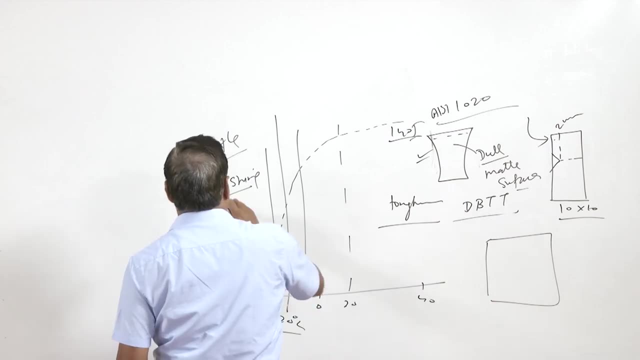 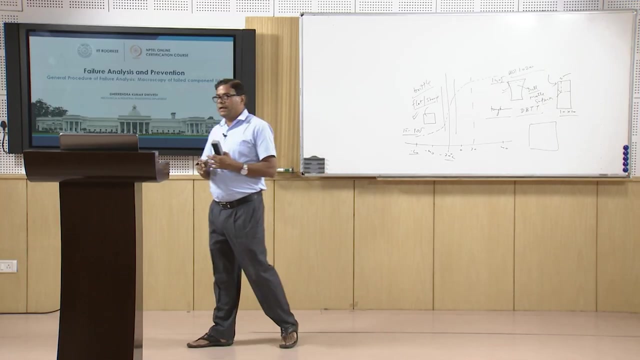 change in the proportions of the fracture. So this involves completely. So this involves completely Shear fracture under the toughness test, and this completely remains, reflects the brittle fracture. So how to indicate that the approximate the proportion of the shear fracture or the brittle 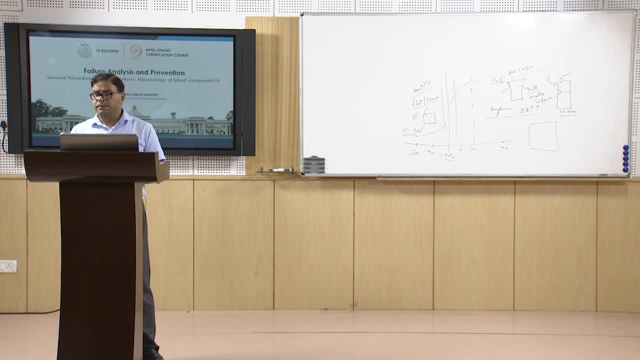 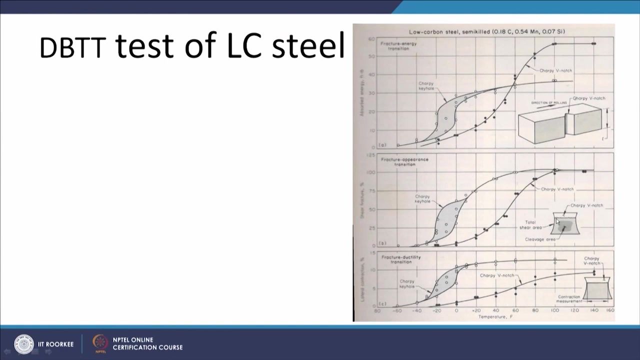 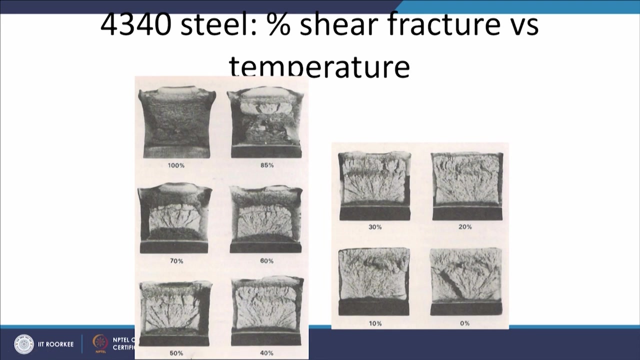 fracture, just by observing the, just by observing the fracture surface. So what we can see here when the fracture takes place. so at the centre we find the brittle fracture and at the sides we find the shear fracture. So how the proportion of the brittle fracture and proportion of the shear fracture change. 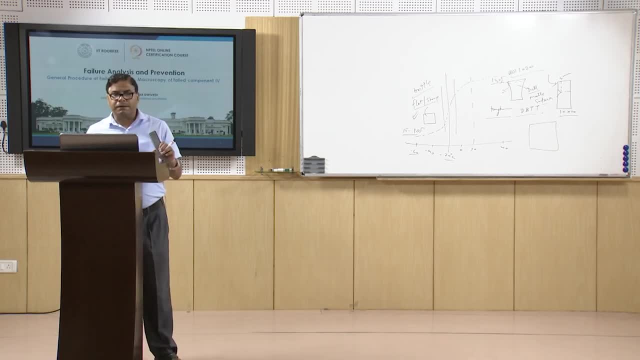 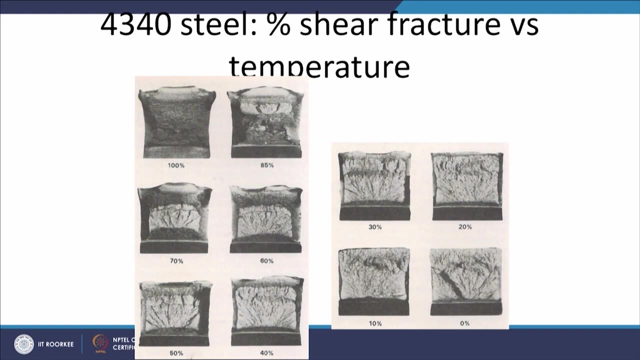 as a function of the temperature. Say the temperature at 40 degree centigrade, it is completely shear fracture. So what we can see here, when the fracture takes place, So the shear fracture and energy absorbed is 140 joule. say just for example this for: 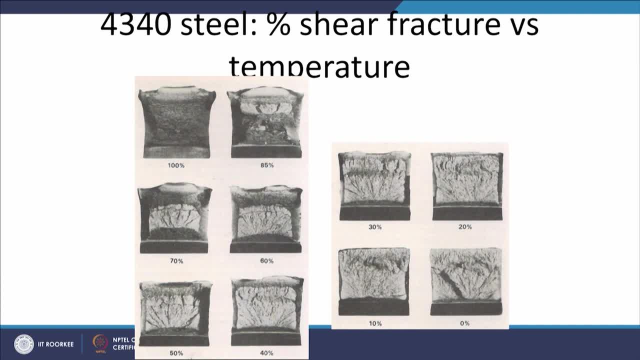 this steel it will be different, like, say, 4340 steel will be. for this steel, impact energy absorbed will be different. But as we move from the high temperature, at high temperature, what we see that it is completely shear fracture. but as the temperature is reduced, what we find that in middle there 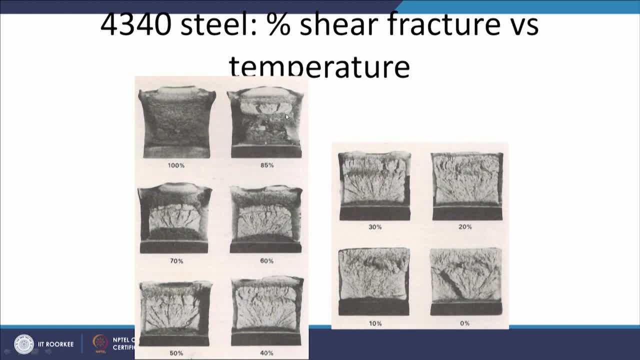 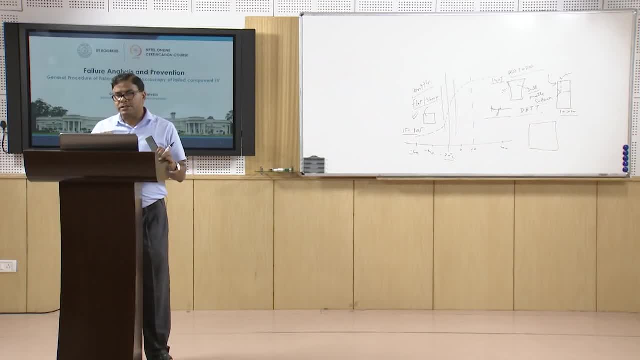 is a brittle fracture which is shiny, And this indicates, in terms of the surface texture and the colour, it is a different from the remaining area. So what is? it indicates that in between it is the brittle fracture, which is about 15 percent, and all around that we have the shear fracture. 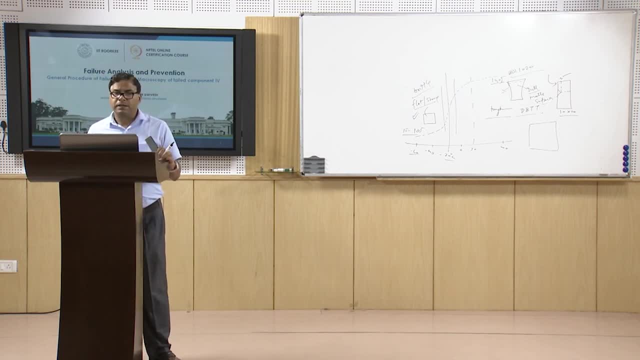 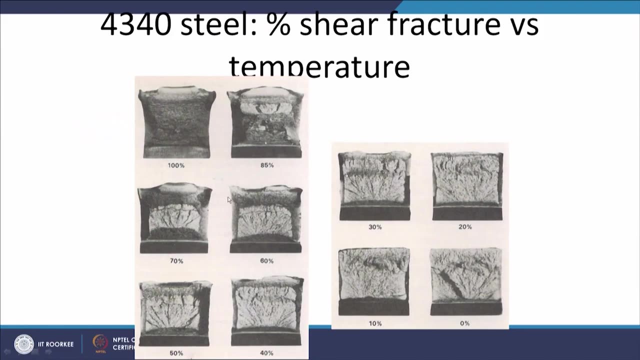 As we further lower down our the temperature, then what we find, the shear fracture is limited to the 60 percent. remaining 40 percent. So this is the shear fracture. So 60 percent is this is the brittle fracture and remaining is the shear fracture. 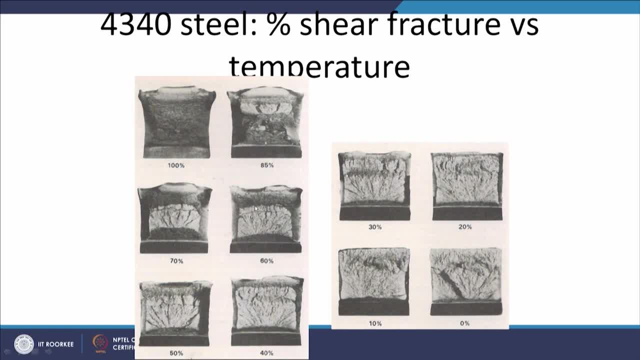 So shear fracture here is 60 percent and remaining 40 percent is the brittle fracture. As we come down for at further lower temperatures, what we see that the shear fracture has been reduced significantly in. brittle fracture has reduced, increased. So in the centre region all this is the brittle fracture. 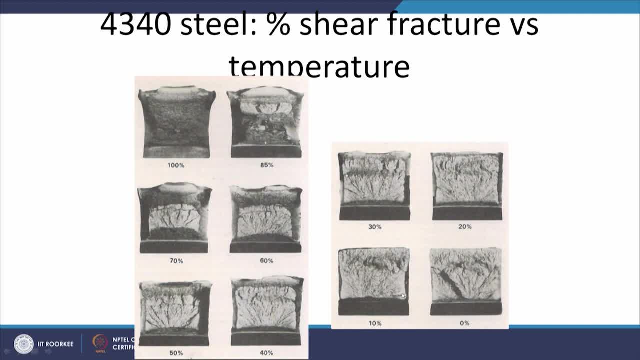 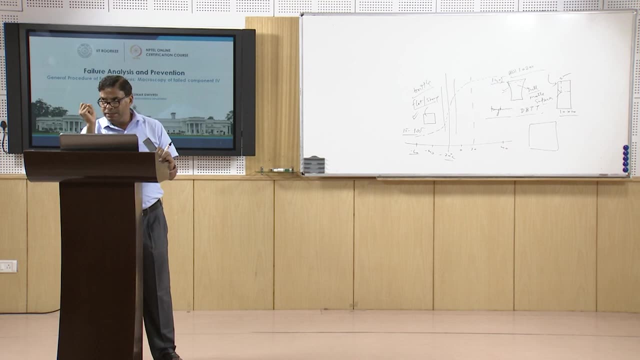 In these two diagrams what it shows? it is almost 90 percent brittle fracture and only 10 percent is the shear fracture, and here it is completely the brittle fracture. So by seeing the texture and morphology of the fracture surface, we can estimate the proportions of the shear fracture and the brittle fractures. 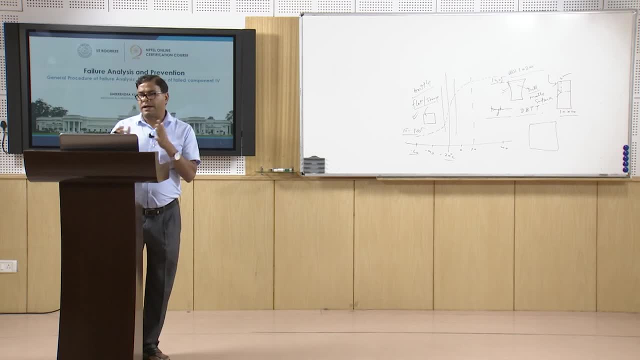 Now we will see that the when the cracks develop Under the different loading conditions, we will find the different morphology of the fracture surfaces. So specimen subjected to the bending on the external surface where the tensile load is acting, it will be showing lot of circumferential cracks. 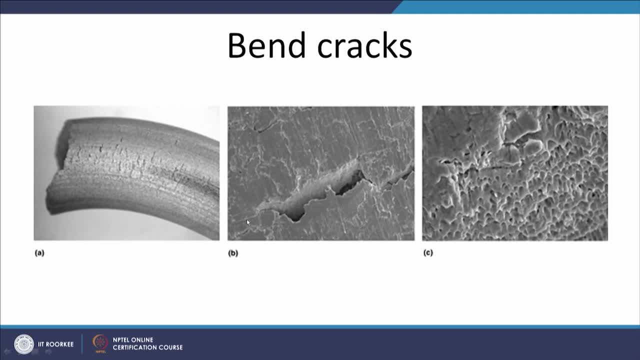 And this is one of the higher magnification micrograph of the such kind of the crack and what it shows? that all the dimples which are present on the fracture surface are oriented, or oriented in one particular direction, that is, the direction of the bending. 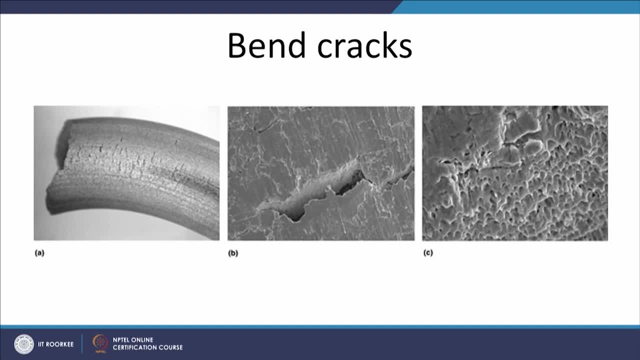 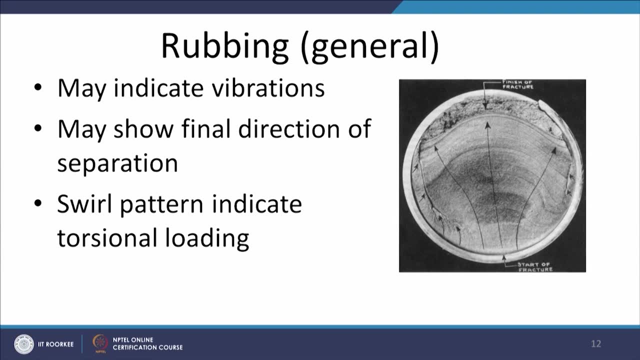 We will see the more aspects related with the microscopic features of the fracture surface in subsequent slides. When we see that the fracture surface is having the rubbing features, so the rubbing features indicate that the possibility of vibrations is there, or rubbing sign also indicates the final direction of the separation. and when the swilled pattern are present on the fracture. 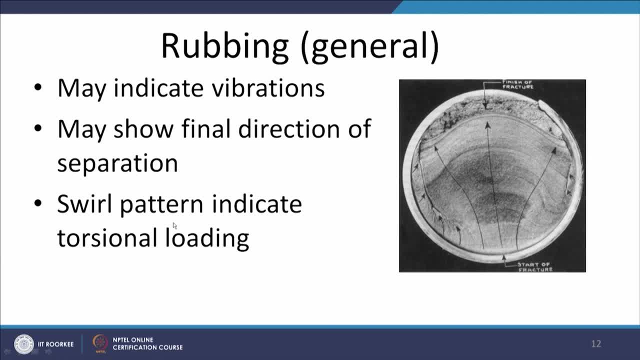 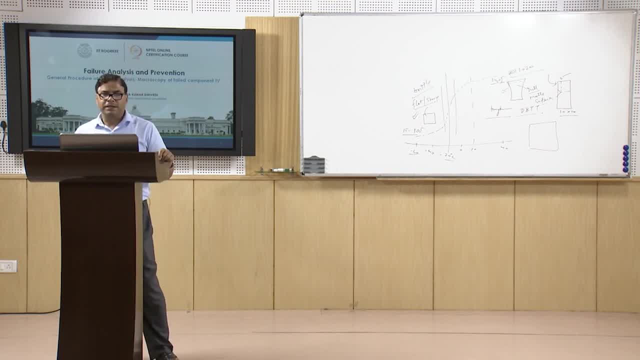 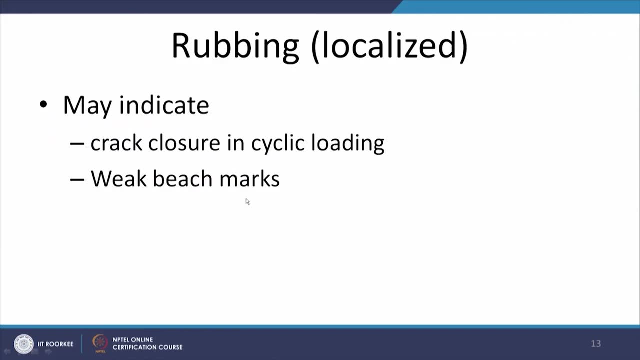 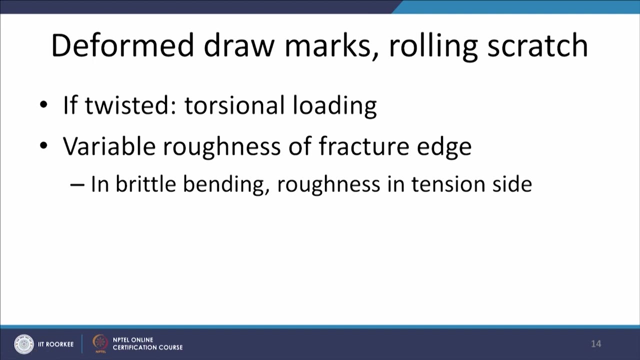 surface, then it indicates the presence of the possibility of the torsional loading. When the rubbing is localized, then it may indicate the crack closure location in case of the cyclic loading or the presence of the weak beach marks. So this component having certain kind of the features like the twisted marks, then it 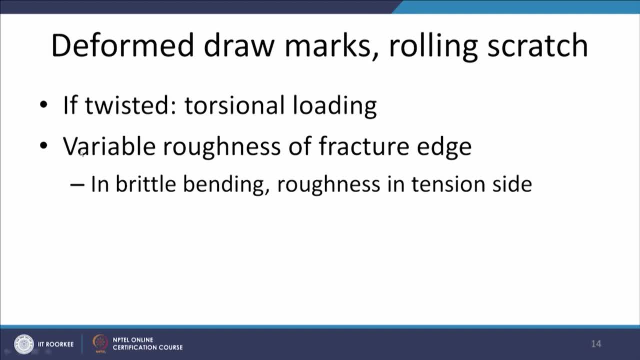 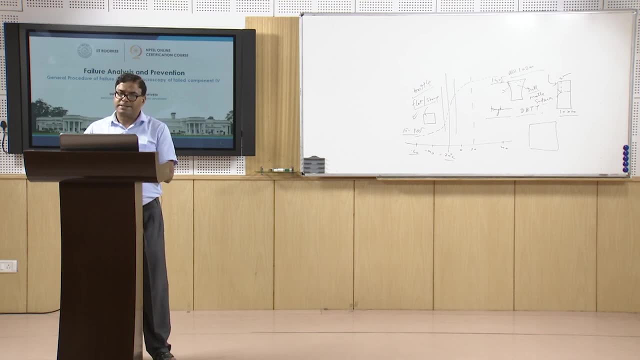 indicates the torsional loading, and when the surface roughness is varying near the fracture edge, then it indicates that in brittle bending conditions roughness is more on the tension side as compared to the other side. So this is how We shall now complete the macroscopic feature aspect related with the fracture surface and 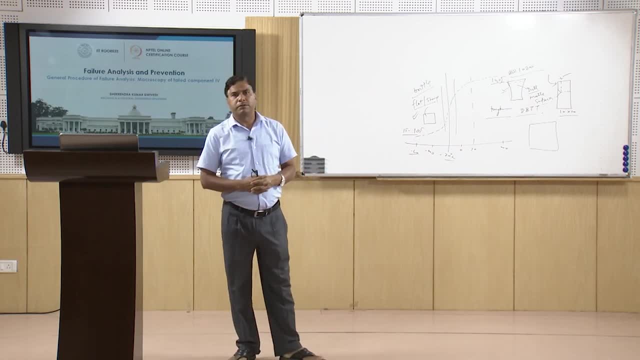 the kind of information which we can gather from the macroscopy of the fracture surface. So in now we will summarize this presentation. in this presentation I have talked about certain additional features related with the macroscopy of the fracture surface, which indicates about the loading conditions, the direction where from crack is initiated and the direction. 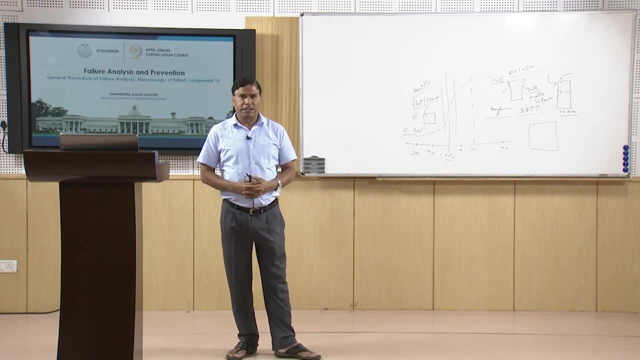 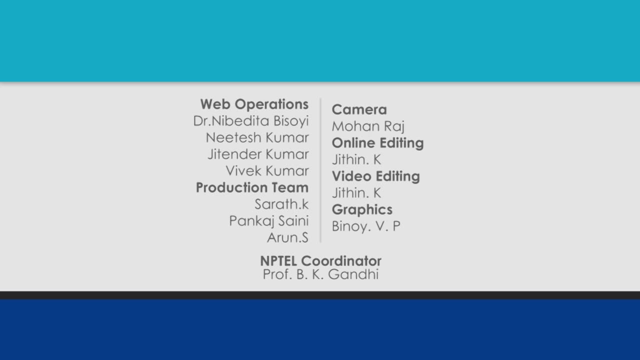 in which crack has grown own. Thank you for your attention.